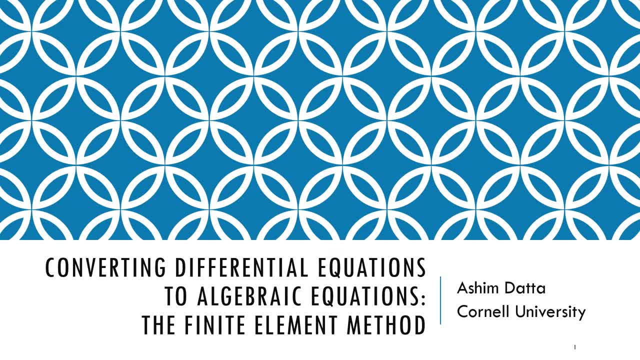 Converting differential equations to algebraic equations is a good idea because it makes the problem simpler and we can solve more complex problems. The finite element method is one of the most popular numerical methods to convert differential equations into algebraic equations, and it is used extensively in 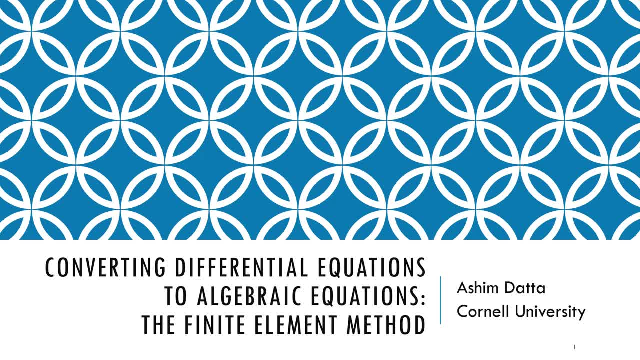 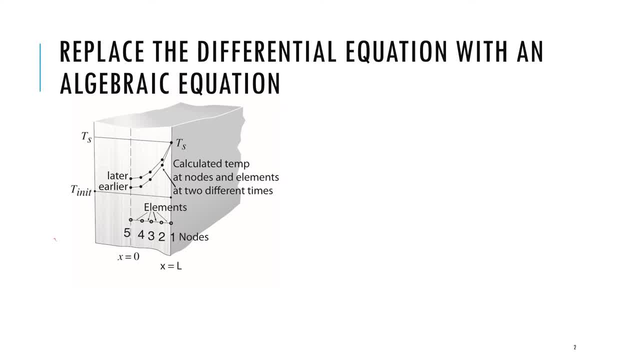 all different types of physics in engineering. So here is our problem. It's heat transfer in a slab, That's this one, and the governing equation is given by the heat equation in one dimension in this case. so the only dimension and the direction we are interested in is is this and so 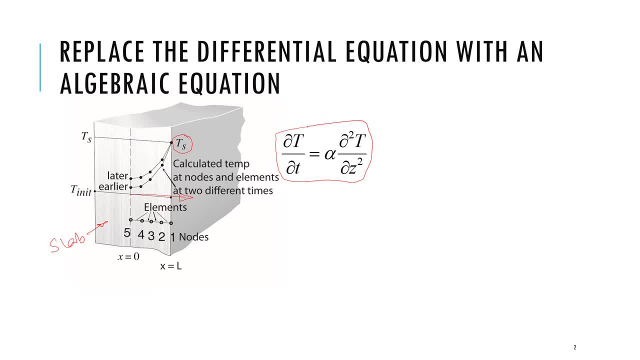 we also have two boundary condition. one can be surface temperature given and the other one is the symmetry. so it's del T, del X at X. equal to zero is zero. so we need to only solve for one half Now in your differential equations. we are going to solve for one half Now in your differential equations, we are. 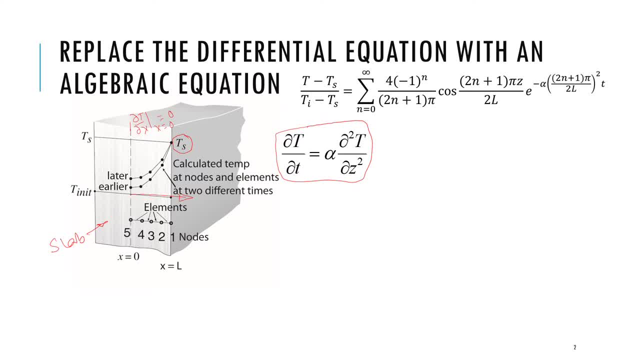 going to solve for one half Now in your differential equations. we are going to: class: you solve this problem and you got an analytical series solution. so class, you solve this problem and you got an analytical series solution. so this is my analytical solution and we are not going to do this one. we're not. 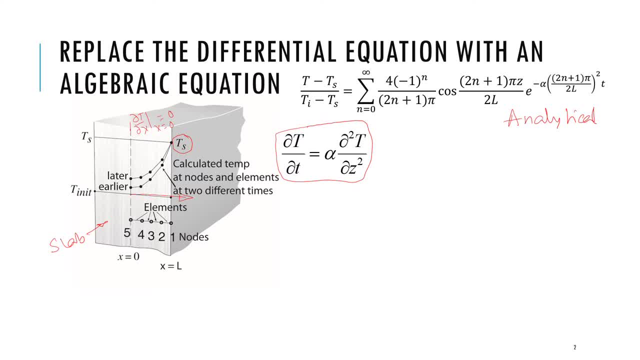 going to use this one because this has a lot of restrictions. so the goal here is we will replace this differential equation with a set of algebraic equation. so this is a matrix, that is, of three equations. okay, and so these are linear algebraic equations where i can easily solve for the three unknowns. now i am showing three as just a representative. it doesn't. 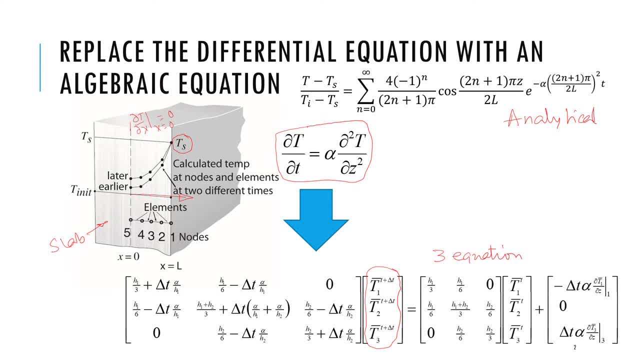 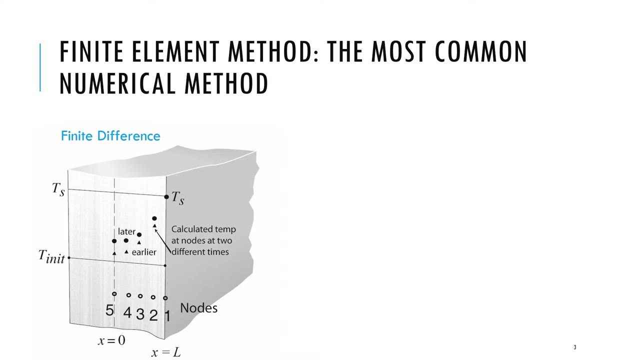 pertain to this particular problem. in reality, you'll have many, many more equations, typically, but the point is you are changing from a differential equation to a set of linear algebraic equations. this is our goal. now most of you know what is a finite difference method, and let's try to compare and contrast. finite element method. 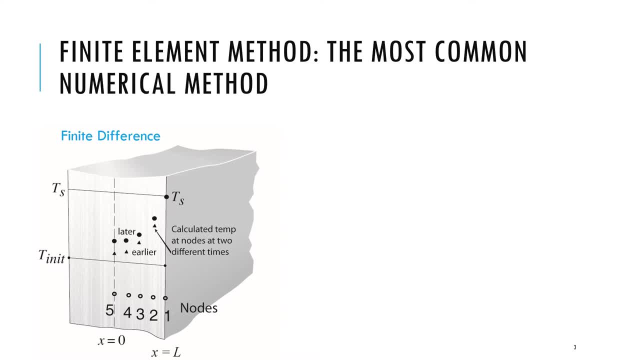 with this simpler method of finite difference that most of you know. so in a finite difference method we divide the domain into nodes and we solve the equation at the nodes to get the solutions. these are my solutions at the nodes. and then, once we get the solutions, then we decide on interpolation in between. 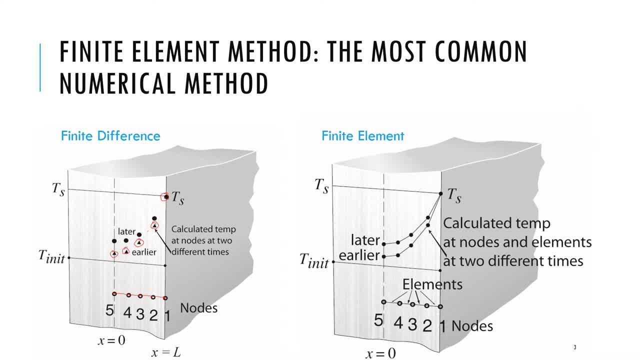 pizza and rien as a final point. so in a finite element method um, it is in a analogous way. it is also that the domain is also divided into the nodes, but here it's not the same nodes, here the nodes and the distance at in between they are together as an element. so nodes andivel. 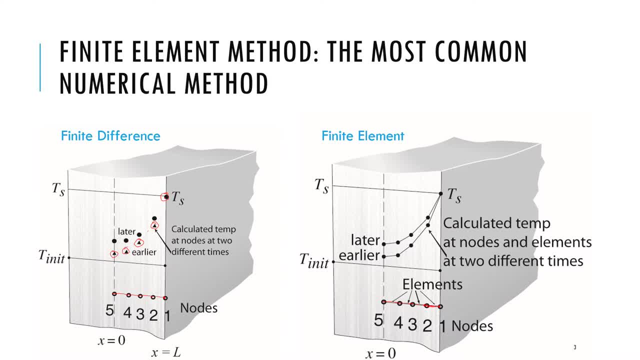 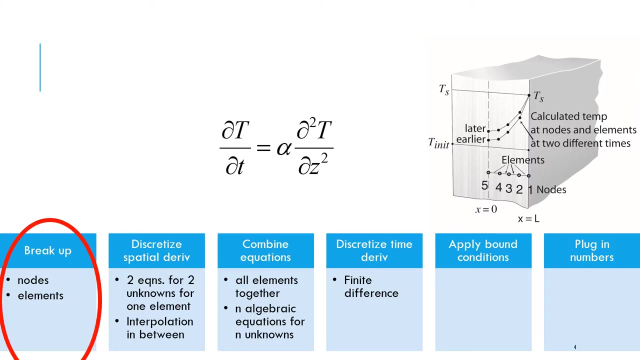 and the distance together, distance in between together, makes an element. but also, when we build the method, the interpolation between the nodes is built in. so, as you can see, the solution is going to be looking like this and this is built into as we develop the method. so now, before we do this, let's have the 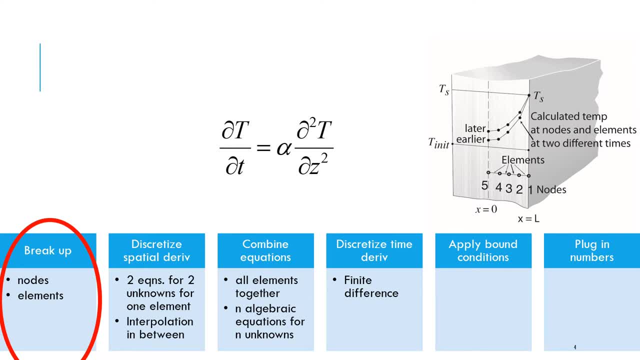 big picture of what we will go through. we will break up the the domain into elements with nodes. then we'll take one of these elements and discretize the spatial derivative- that's this one, the spatial derivative- and then we combine the equation for all the nodes. then we discretize the time derivative and then apply the boundary conditions. 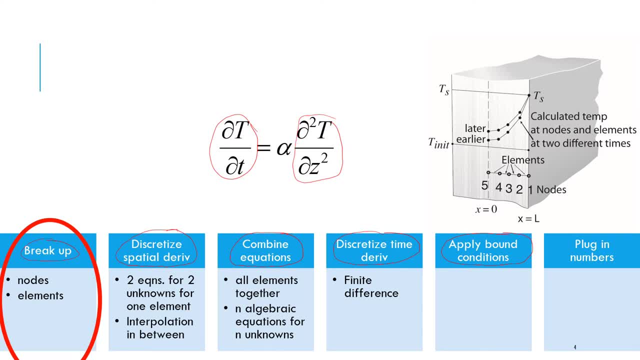 and finally, just to make ourselves feel comfortable, we'll plug in numbers. so that's the step we're going to go through. so first is breaking up into nodes and elements, and so this is a 1d problem. so this is my domain and I am going to break this. 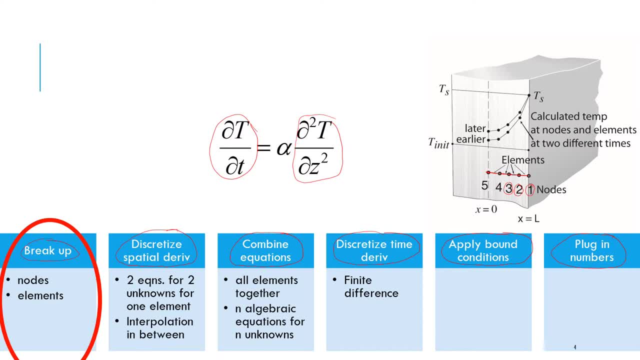 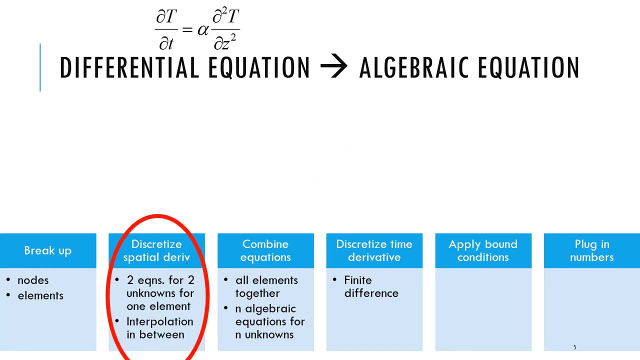 up into five nodes. that means four elements, four elements and five nodes. and now we're going to work with one of these elements. we will discretize the spatial derivative- that's this one- and convert it from a differential form to an algebraic equation for one element, and we're going to do that for one element. so for one element, it has two nodes. 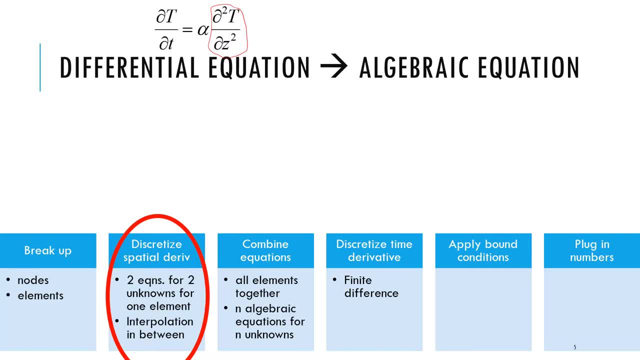 so there are two unknowns and our goal is to get the two algebraic equations. we will do this using three steps, so first we assume a straight line solution between the two nodes and then minimize the error to get the two needed equations. okay, so we'll go through these. 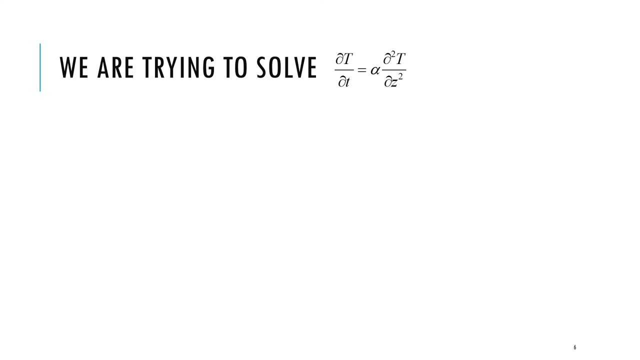 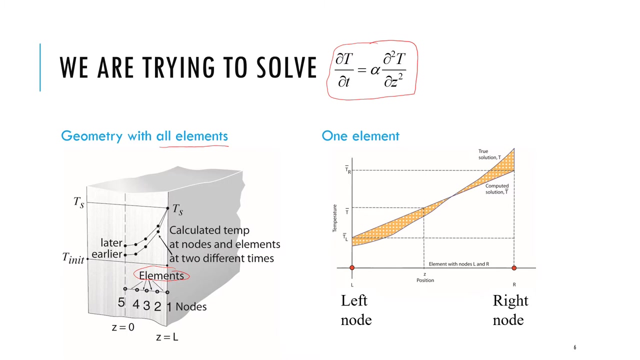 steps now. so again we are trying to solve the heat equation. and here is the geometry with all the elements. these are the elements here, and on the right we have enlarged one element, so let's say between three and four. this element we have enlarged, so this is like four, and then this is like three. okay, so 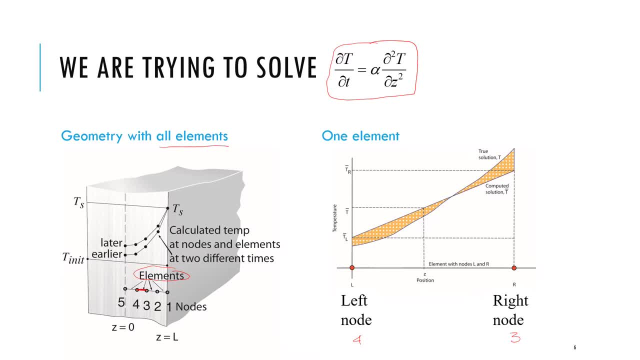 for this element. we have the unknowns as the temperature TL bar on the left node and then TR bar is the value of temperature at the right node. these are unknowns, these are what we are trying to solve for. so these are unknowns. and in between TL and TR there is a linear interpolation. 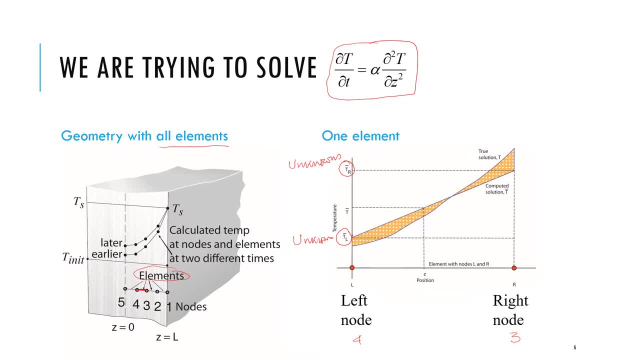 so values in any location in between can be found by simply linearly interpolating. so now this is my solution that we are trying to compute. I have superimposed the true solution, which, of course, is an unknown, but I have super imposed that in there, that just to contrast what we are. 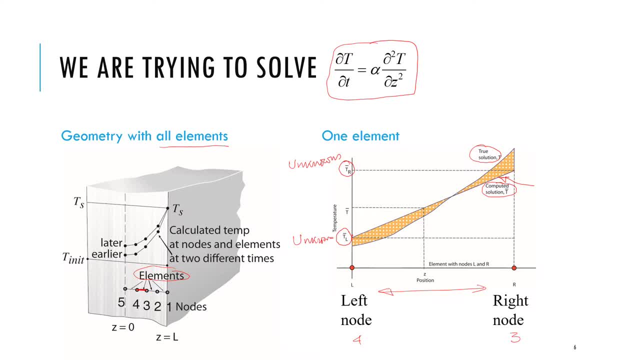 going to compute with the true solution, which is an unknown. now. there is no reason that this solution, that we have a value in between that is going to be lying down here and over here. the C was Winchford and now we have the three and we are going to compute which would be some sort of approximate solution, would be exactly equal. 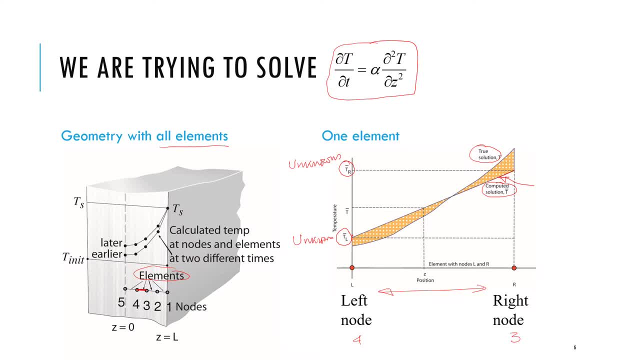 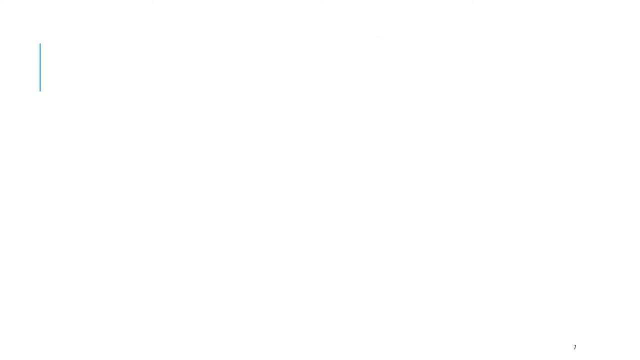 to the true solution? in general they will not be. so the shaded area- this shaded area- that's the difference between computed solution and the true solution- is the error. this error can be positive or negative. okay, so now we try to minimize the error to get to the needed equation. 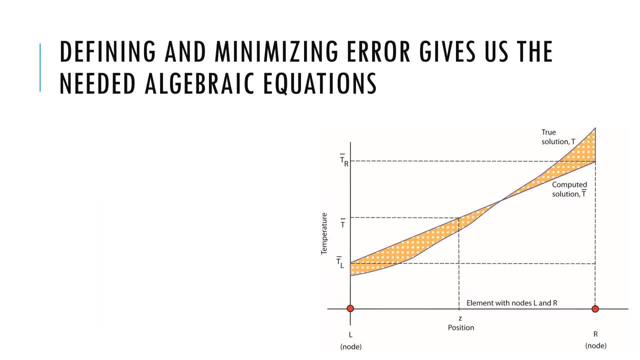 this is the sort of the second step. so again, the true solution is something we do not know. we will only compute an approximate solution- t bar. so we will only compute an approximate solution- t bar. so we will only compute an approximate solution- t bar. so the error is this shaded zone and let's see how we can write this. so the true solution 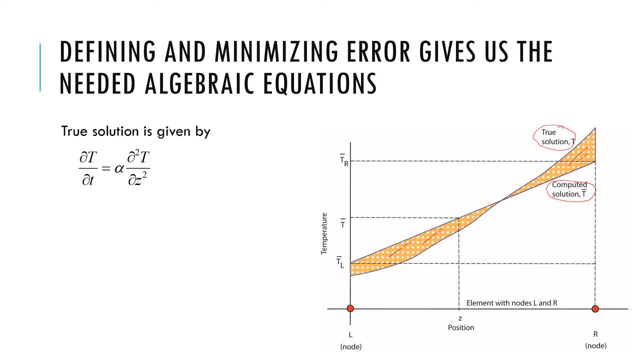 is given by, of course, the my differential equation and t bar. the bar is for approximate solution, so t bar is an approximate solution. so the error, that's the shaded, of course the error that's the shaded zone is given by the difference between two. so if they are exact then it will be zero and my this equation will give back my. 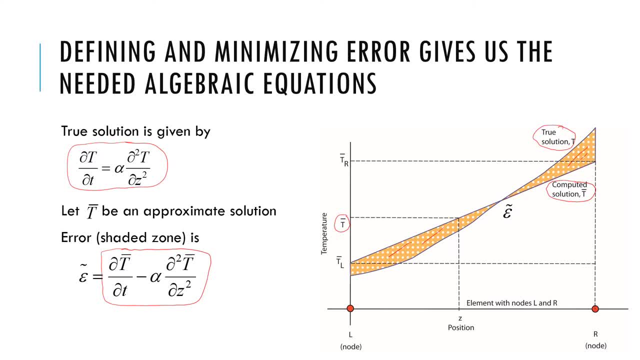 equation that i started with: okay, otherwise, in general it will not be zero. so this epsilon tilde is not going to be zero. so this epsilon tilde is not going to be zero, and so we want to make this error zero on the average. now, if we just do, 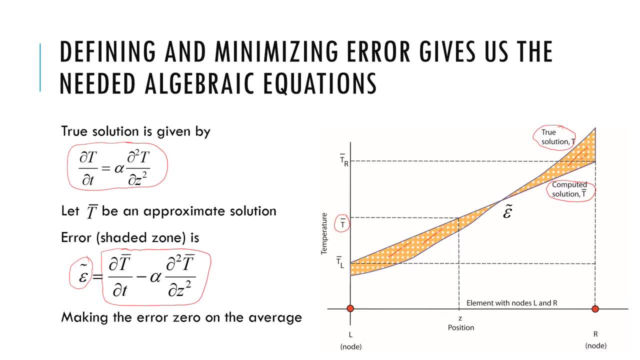 the average, meaning we add up all the errors here and here and set them equal to zero, which would look something like integral epsilon, tilde dz equal to zero. this is not a good idea because then we could have a lot of negative error and positive error together. it will give zero. 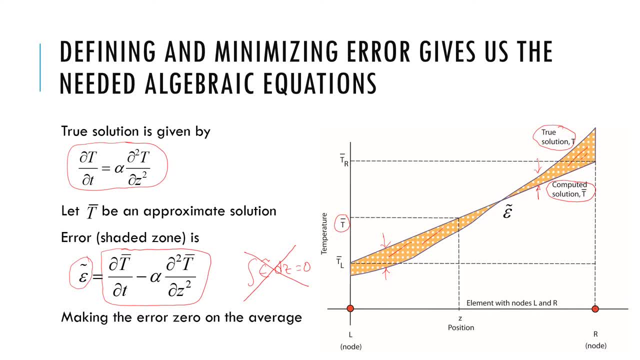 but there will actually be a lot of error. instead, we use this weighted average, so the weighted average looks something like this. so, instead of just epsilon, tilde dz, we multiply by these weights until we add up two terms and it looks like this. so, for example, we will increase or decrease. 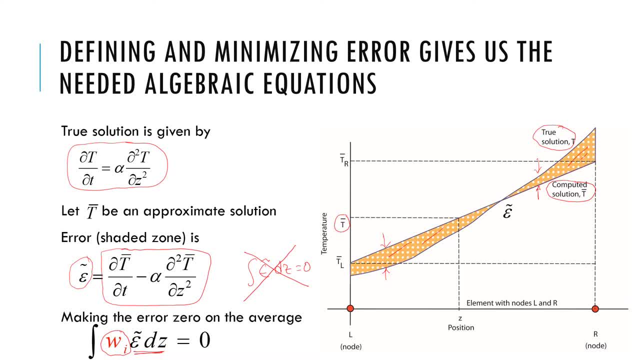 weights. we will soon discuss where the weights come from, but it's important to note- very important- that error is not made zero at every location, so we're not going to have a solution. this is what we are going to have, that we will match at every point. this is not possible, so we will have to. 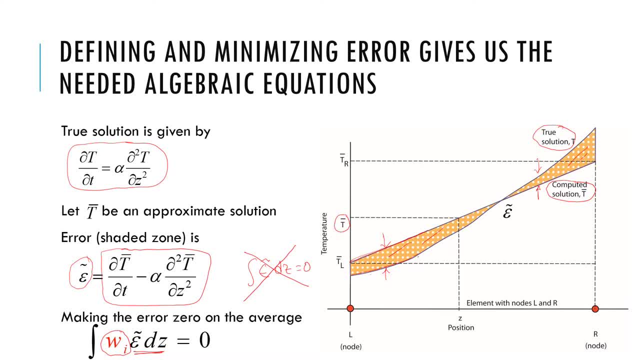 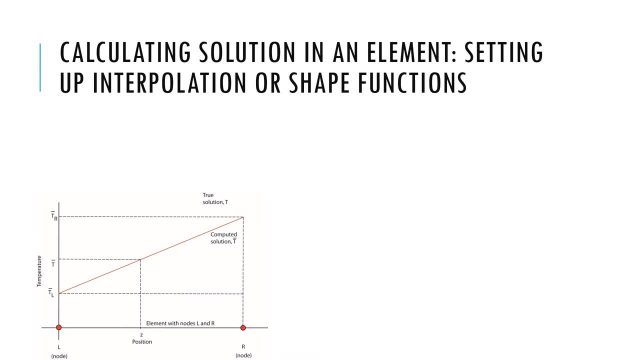 accept some error. this is the fundamental source of error in this kind of numerical computation. before we get into the weights, we just develop the equation for interpolation. this is typically something we do in high school. so this we just want to have an equation to this line. so let's write this from these two similar triangles: 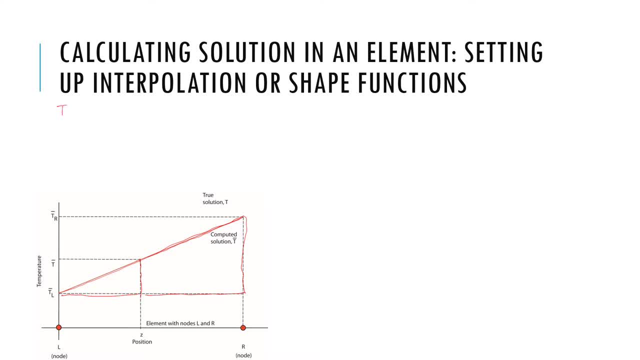 i can write a t bar minus t bar is any temperature t bar here at position z, and so i write t bar minus t l bar over z minus l is equal to this part, which is t r bar minus t l bar. this total distance r minus l. okay, so this i can simplify as t bar is equal to t l plus z minus l. 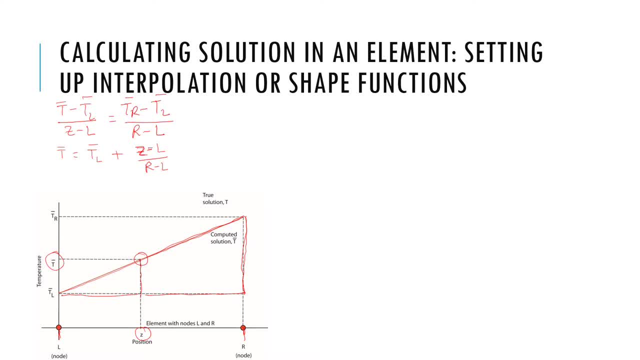 over r minus l times t r bar and t? l bar bar. and further simplifying putting the t? l's together: t l 1 minus z minus l over r minus l times t l bar plus z minus l over r minus l a t r bar. and so if i just do the subtraction, 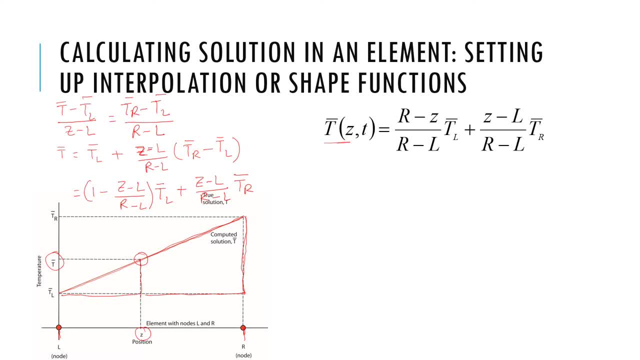 i'm not going to need a bunny spaceman, right. i'm just going to have to do one more step. so lets look at the intervention. what is this? the right value, depending on where you are? okay, so we can write this in for just just making things. 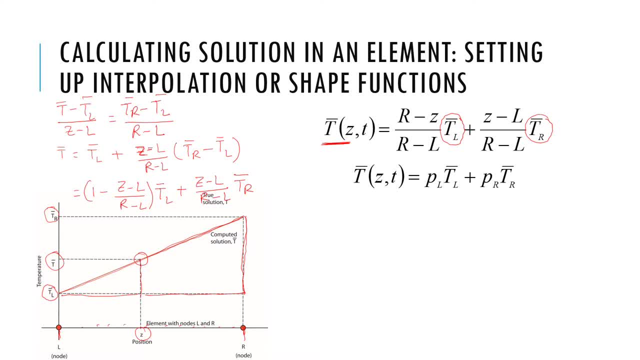 simpler in terms of doing the algebra. we can call this part as pl and we can call this one as pr. why pl and pr? because in general, in a much more complex finite element development, these would be polynomial of other order. so here it's: it's just a polynomial of degree one, it's just pl. 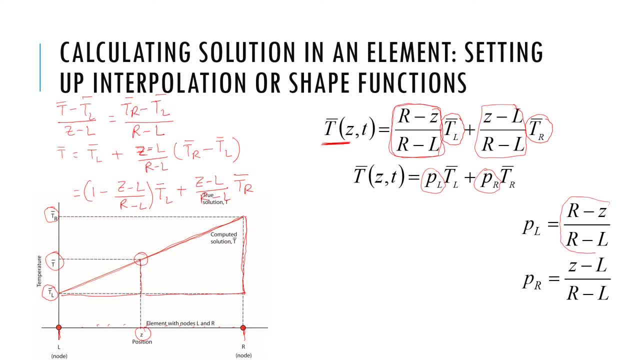 is equal to r minus z over r minus l, and p? r is z minus l over r minus l. so they are just really equations for line and so if I plot these they look something like this: so pl at z equal to L, it is 1. 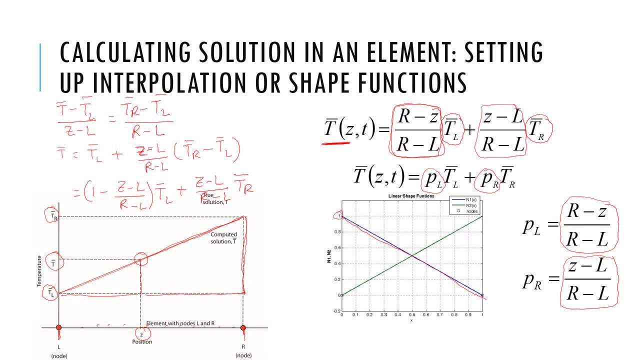 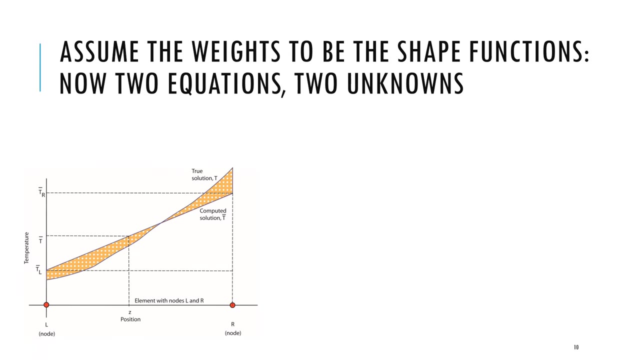 and so it goes from 1 to 0 and pr goes from 0 to 1. so polynomials are also called the Lagrange shape functions, which we don't need to get into any more details. so back to the definition of error. we want to make the error, that's these: it to be 0 on the average. okay, so this gives me a. 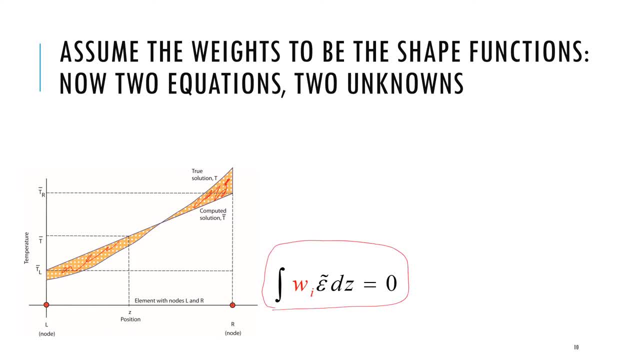 okay, so from L there goes the value 0 and p, and then the P, and so we can further study this деfinition. we want to use this equation and then we want to use two different weights, the two next to Xètres polynomials that we just defined. 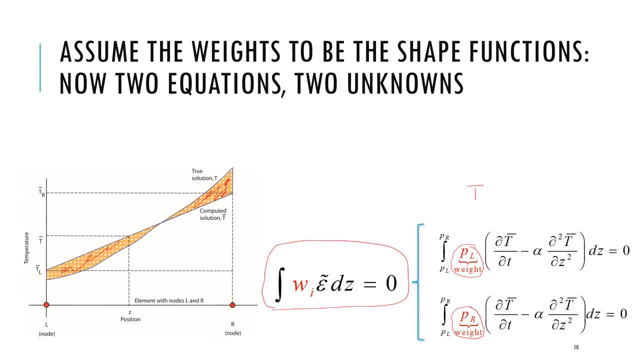 that we solve these two equations for the two unknowns tl bar and tr bar, which are the only two unknowns for one element. so elements have two nodes and those two nodes are the, these two unknowns, so two unknowns. to solve for them we need two equations, and these are the equations. 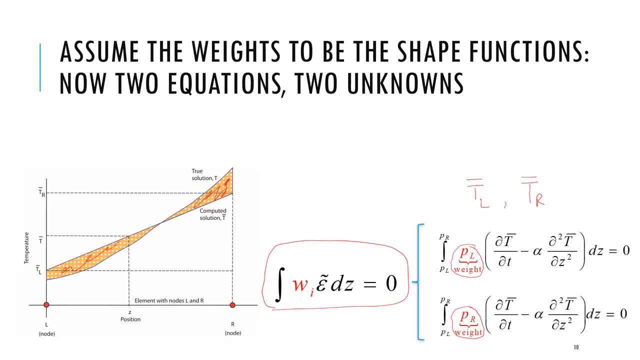 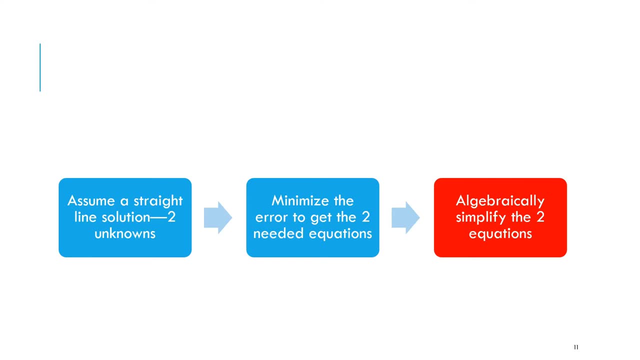 and the way we got the equations was my make, by making weighted average of the error to be zero. so the last part is to algebrically simplify those two equations. it's nothing, but you know very simple integration and stuff that you did in sort of the first. 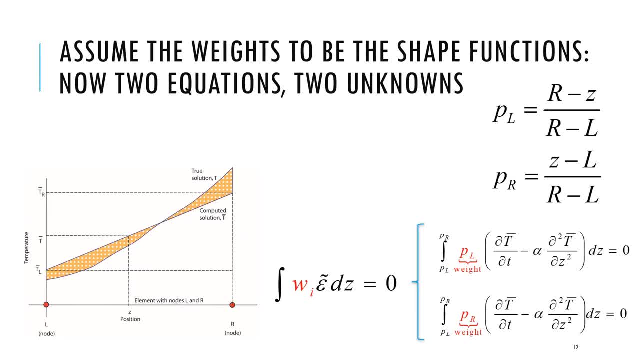 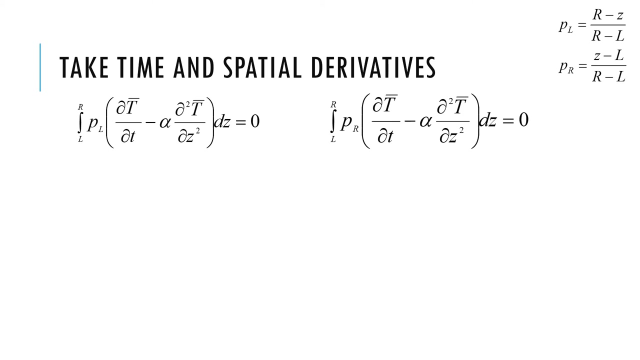 course in calculus. so to repeat, then we're going to plug in this pl equal to this thing, we will plug in in here and we will simplify the equation. likewise we will plug in pr in here and then we will simplify the equation. so those two equations again, and we're going to substitute for pl, pr, but we are also going to substitute for the. 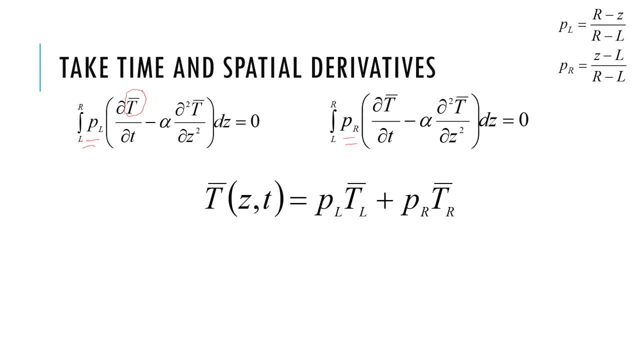 the temperatures using our approximate solution. so our approximate solution is this: we will try to find this tl and tr and then in between at any location we will interpolate. so the this is my approximate solution. so this also needs to be plugged in to both of those terms. so 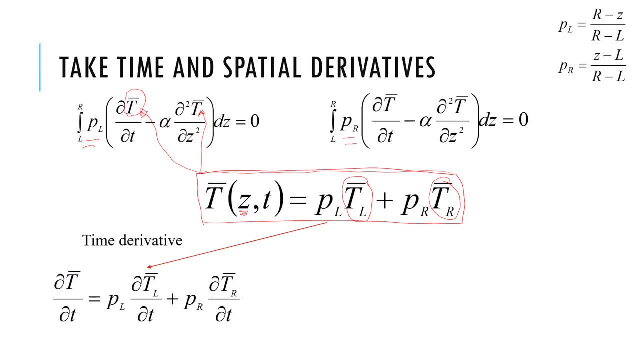 let's see how we do that. so for the time derivative, then you notice that pl here and pr, they're not really functions of time. they don't change with time. so if i take the time derivative of the solution, then pl comes out and we get del t, l, del t and del tr, del t. so t, l, t, r are the nodal temperatures. 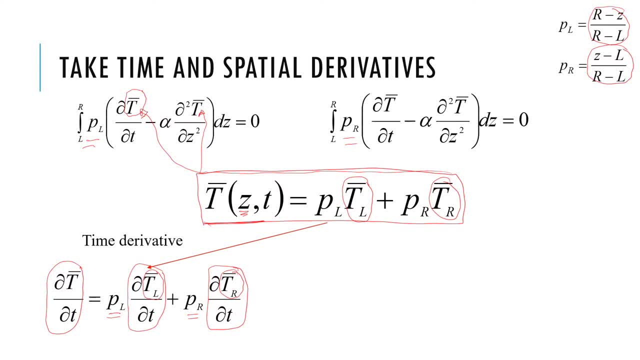 that will change with time. um, so the spatial derivative. on the other hand, i can write del, t, del z as t l bar. it comes out t? l bar is the temperature at that location, so it's not changing with with location. that's the temperature at the fixed location and then p? l, as you can see. 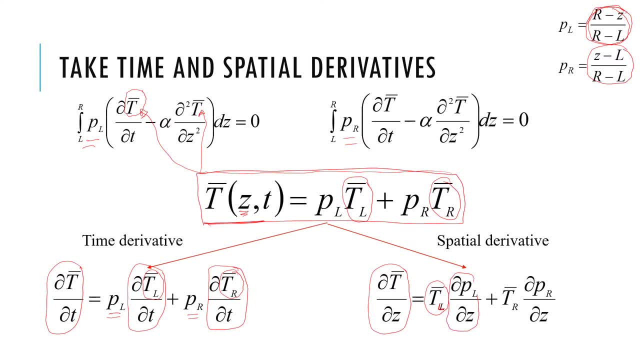 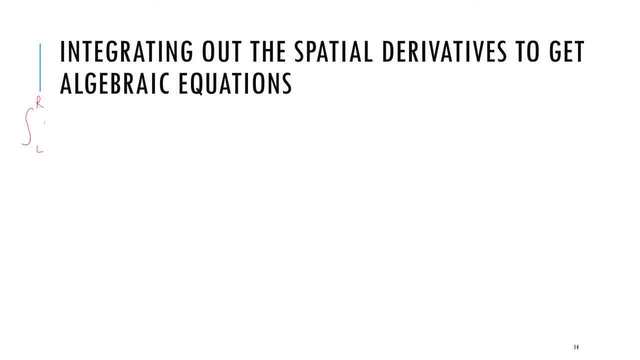 it is a function of z, so i can write del p? l del z, likewise for t? r bar and del p? r del z. so basically we want to plug in things into this equation del t? bar del t minus alpha del square t bar del z square dz equal to zero. we want to plug in here two things. one is pl equal to. 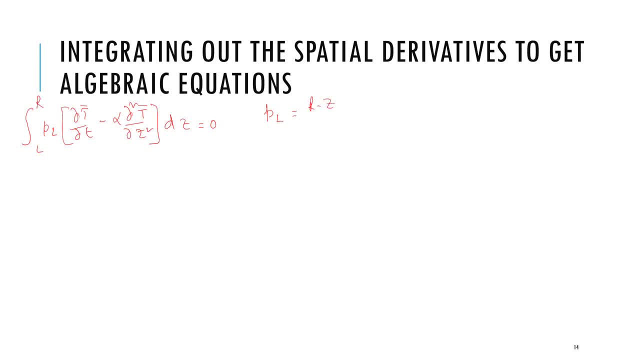 um r minus z over r minus l. and also t bar is equal to p? l t l bar plus p? r t r bar. we just want to plug in both of these into this equation and simplify. that's all we're going to do, okay, so, um, if i plug in for t, 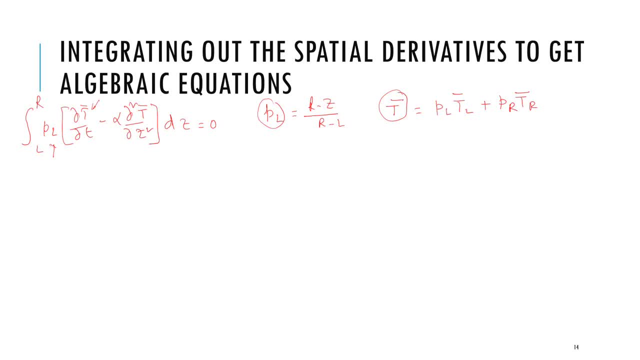 then, as we already did in the last slide, the del T bar del T is going to be PL del TL del T plus PR del TR del T. this is the trouble of using PowerPoint is we are repeating some of it. so if I plug that, plug this term in here. this is the. 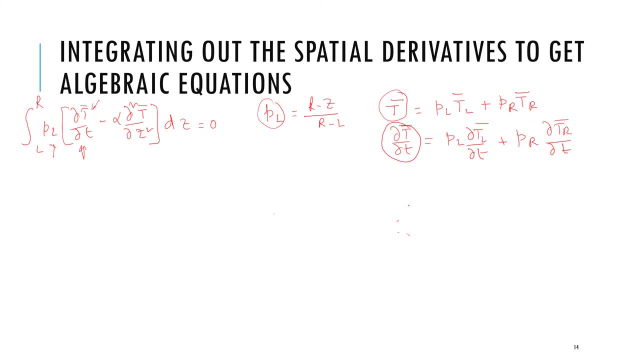 term that we plug in here, and PL, so integral L to R when you plug this in, because del TL, del T is not a function of Z, so that comes out okay, and we get PL from here, from here, and then another PL from here, so it's PL. 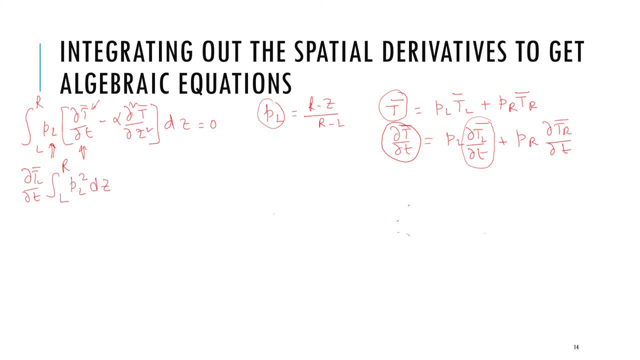 square DZ. that's the first term, and then the second term would be a plus del T, R, del T and integral PL PR DZ. okay, so that those two just comes from the first one, this one here and then the next one is minus alpha PL del. 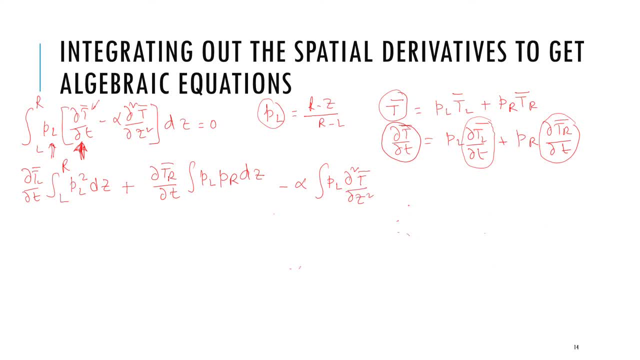 square T, bar del Z. square DZ. again, it's all between L and R. is it equal to 0? so this second term is kind of troublesome because we don't have something for the second derivative. so let's see what we can do. okay, so to. 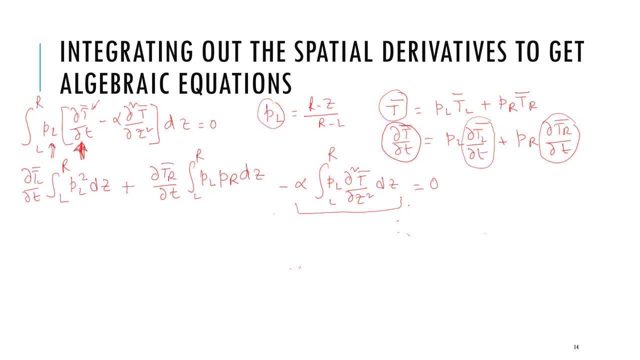 convert this second term. you see I can write: del del Z of PL del T. bar del T Z is equal to a PL del square T bar del Z. Okay, and so if I bring this guy that I need to the left hand side, PL del square, t bar del z? square is equal to del del z of PL del t bar del z minus del p l. 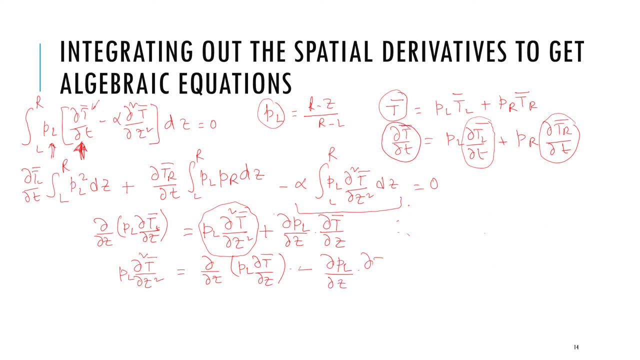 Okay, and so then, if I integrate both sides- so now I integrate both sides, from L to R- then you see, this is the term that I needed here, This is the term that I needed here, And So I now Do that. 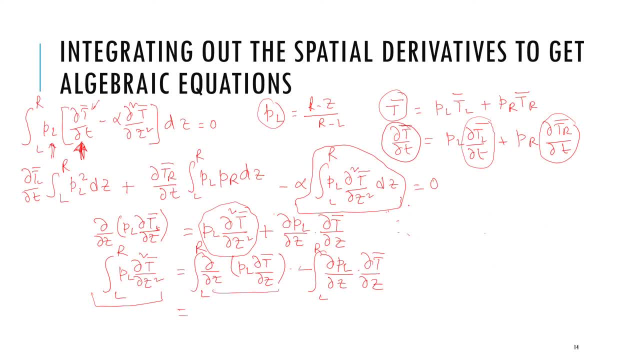 I integrate out this one And so this gives me PL del t bar del z at R, because it's del del z integrated over del z over DZ. So then I get back this function at R and then minus at L del t bar del z at L. 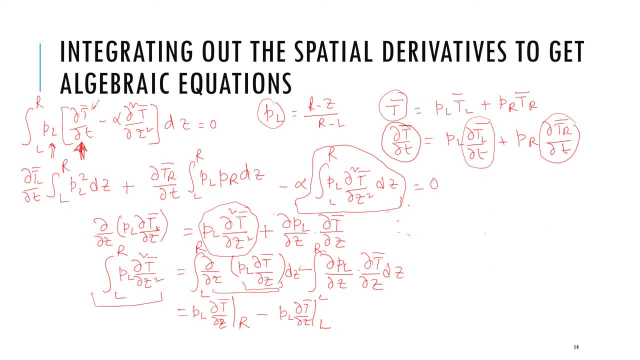 And then For this one, It's Del PL del z, Del PL del z. I can write from here as a TL del PL del z plus TR del PR del z. Okay, DZ, Okay, I can write this as a TL del z minus TR del PR del z. 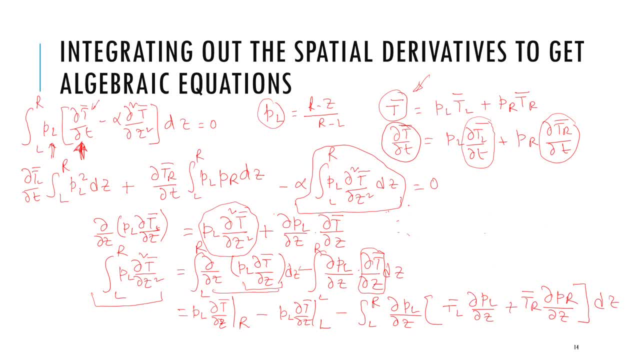 Okay, And so Now I'm going to write this as a TL del. I can write this as a TL del. I can write this as a TL del PL del z plus TR del PR del z plus TR del PR del z plus TR del Z. 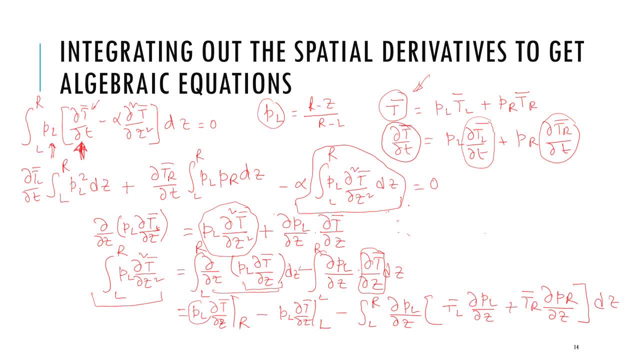 Now you see this guy, PL at R Is zero. If you look at this, PL at R is zero. So this first term goes away. So it's the next term minus PL Del T, bar Del Z at L minus. then here we see it's: TL bar integral del PL del Z, squared a DZ. 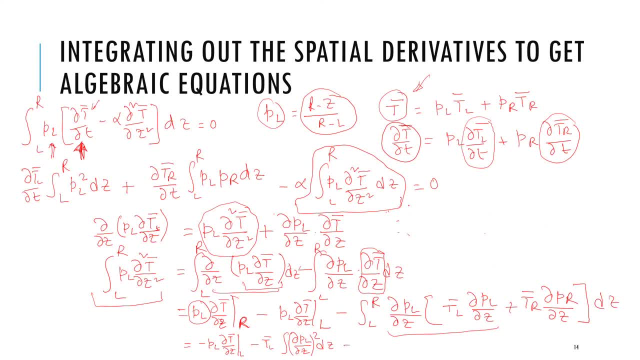 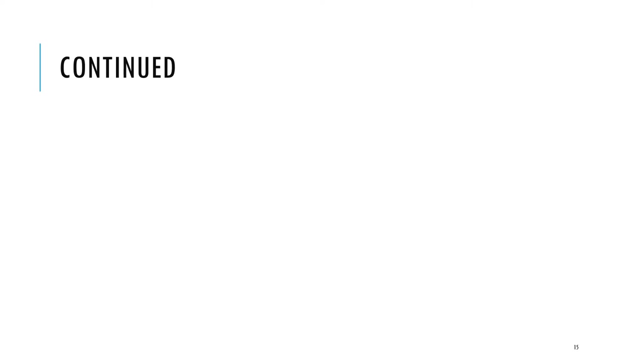 minus TR, bar integral del PL, del Z, del PR, del Z, DZ, L to R and also L to R. that's as much as we can put it on this page, so let's stop here. okay, with the limitations of PowerPoint. unfortunately we have to rewrite some of. 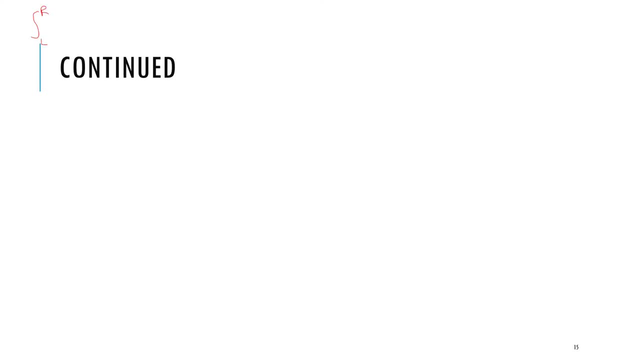 the stuff. it's so the equation that one of the two equations we got for solving for the left node and the right node is this one: PL a del T, bar del T minus alpha del square T bar del Z, squared a DZ equal to 0. this is one of the two equations and we were plugging in for PL. 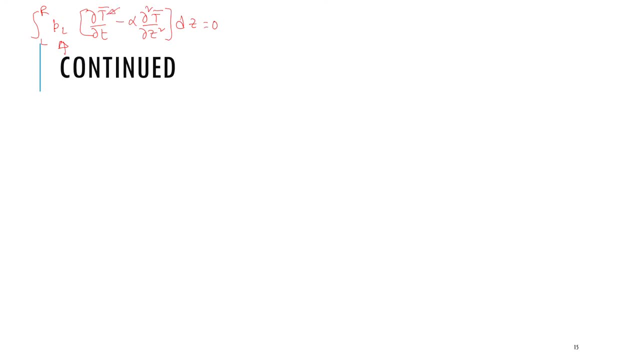 and T bar, but we only have plugged in for T bar so far and from there we got this equation del TL, del T, integral PL squared DZ. so this is what we got part way plus del T bar, the TR bar, delt and PL PR D Z L to R, minus Alpha PL del square T bar, del Z square D Z L to are. 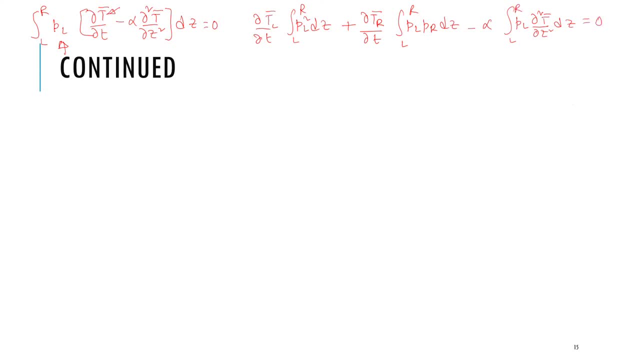 equal to zero, And then we just spent quite a bit of time trying to simplify this term. So the final equation we got there is del TL del T PL square dz plus del TR. bar del T L to R PL PR dz plus alpha Alpha PL. this is the part that we just did. I am substituting that del T bar del Z at L plus TL alpha L to R del PL del Z squared dz. 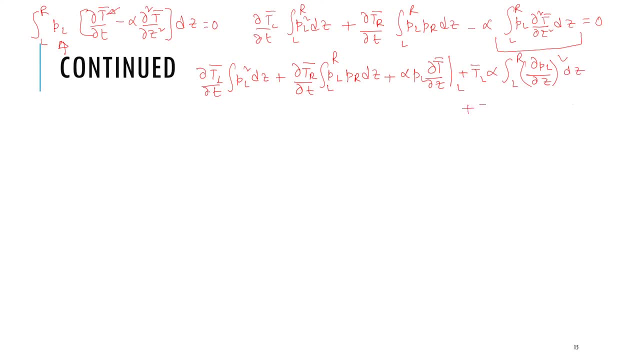 plus TR, bar Alpha and L to R del PL, del Z, del PR, del Z equal to zero, So where I simply have substituted what we derived in the last slide for this term. So we got this equation. So this is one of the two equations that we'll solve to get TL bar. 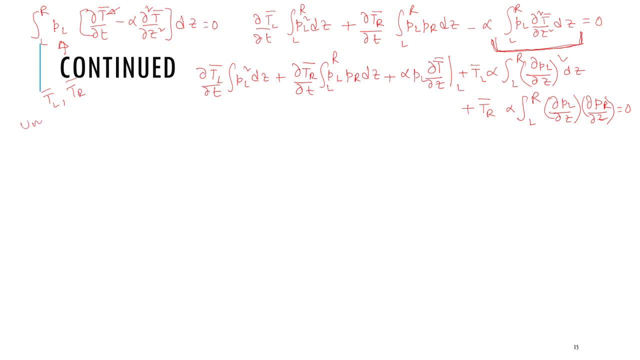 And TR bar, which are my unknowns. Okay, so let's not forget that. So now notice. it has all of these terms like this: But what is PL? PL is simply Z minus R over L minus R, So R and L, they are constants. 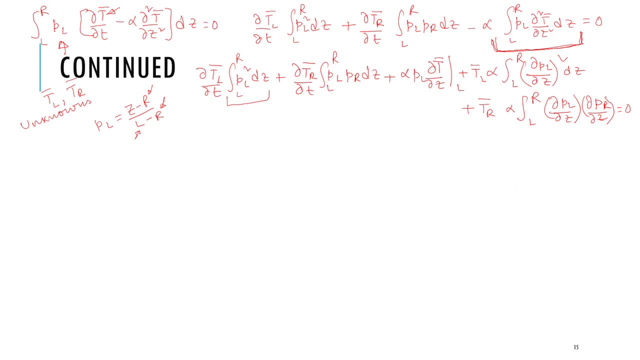 So this is a simple equation. So let's do one of these. So let's do PL square dz, L to R, which is equal to Z minus R. square over L minus R. square, plugging in for PL, Okay, And dz is equal to L minus. 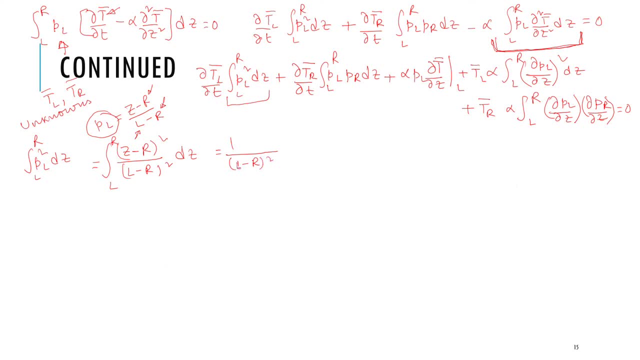 And then integral L to R Z square minus 2 ZR plus R square dz, And let me try to clean some of these. It is equal to 1 over L minus R, So 1 over L minus R square and the integration of this will give me Z cube over 3 minus Z square R plus R square Z between L and R. 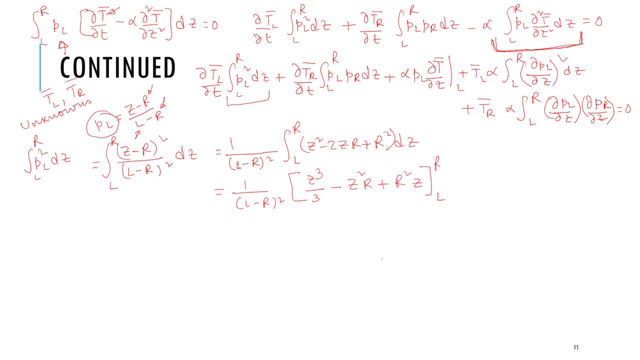 And so that if you plug all these in- Okay, let's do one of these- 1 L minus R square And you get R cube over 3 minus R cube plus R cube. As I plug in R, then I plug in L minus L cube over 3 minus L square R plus R square L. 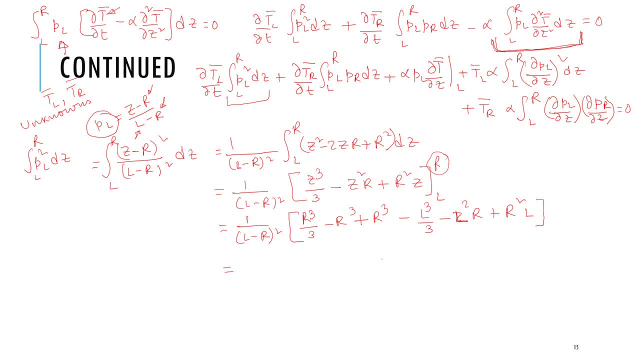 And that's equal to 1 minus L, minus R square times. If I take 3 in the denominator, Then I can write R cube And minus 3. L square R, and so minus 3 L. Yeah, So minus 3 L square R. 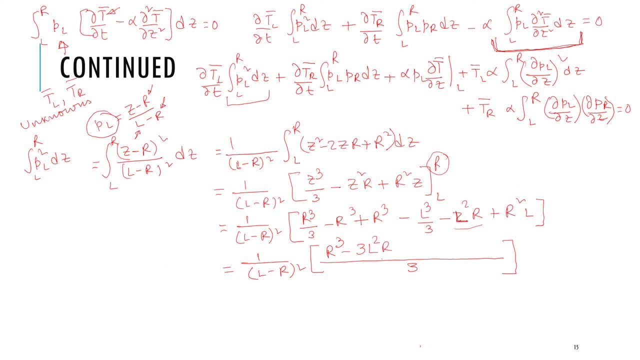 That's this term here, Sorry about that. Plus 3 R square R square L and minus L cube, and these two cancel out. So if you recall this, the numerator inside the bracket is L minus R cubed. Okay, over three. 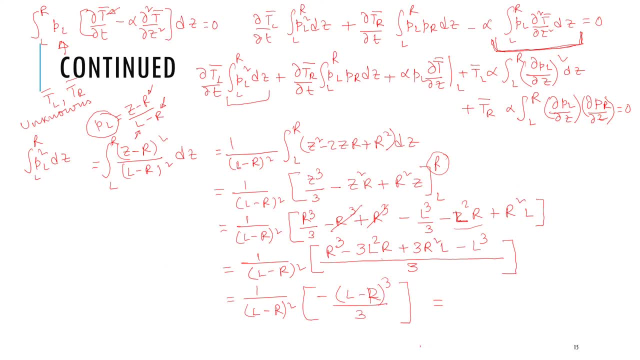 Okay, so this is then equal to Minus L minus R over three, equal to R minus L over three. So this term, you notice, even though you know it's a square, Well, it's a perfect square. Let's say we have this: 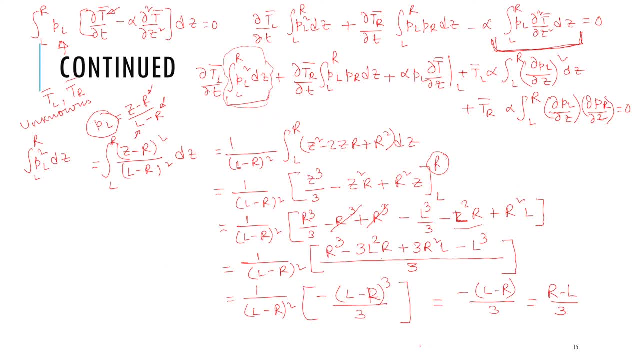 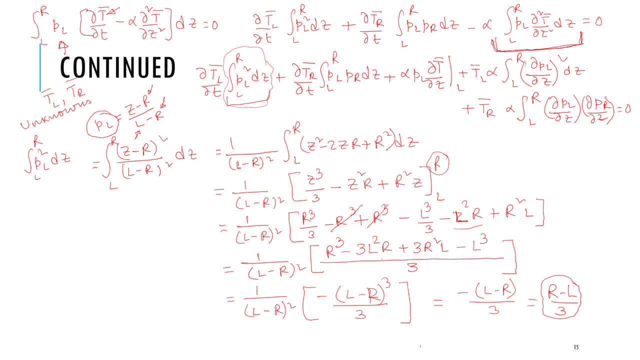 point, that is that has to be made now, instead of going through all of them. I want you to see that these terms like this can be integrated out and and you will have a simple value like this: R minus L is simply the length of the element. so, in case you you don't believe me, let's do another term that looks: 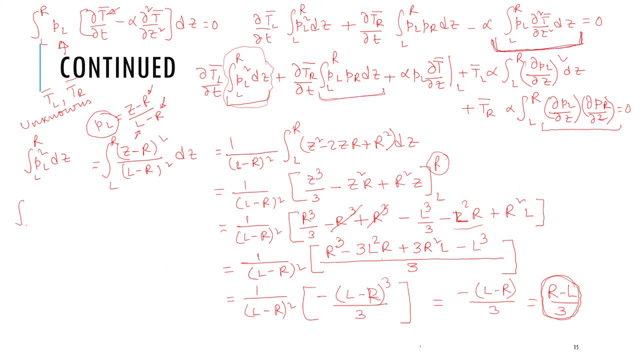 quite different. so integral L to R and just trying to keep things separated: L to R, del P? L del Z, del P? R, del Z D Z, and that is equal to L to R. what is del P? L del Z, del P? L del Z? if you look at this expression del P? L del Z is just one. 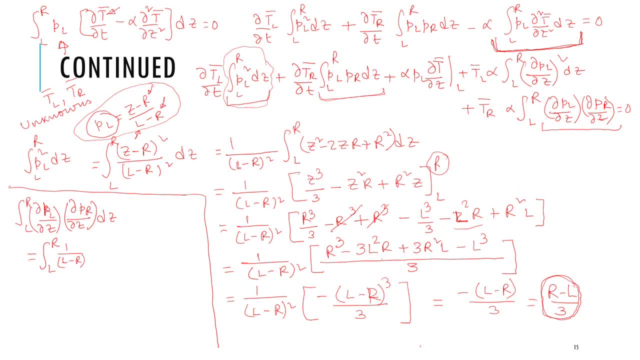 over five L minus R, okay, and similarly del PR, del Z. if you plug in for PR, then you get R minus L a DZ, okay. so what is that? equal to? that's equal to. that's equal to minus L, to R, R minus L square DZ, which is equal to minus R minus L. if we 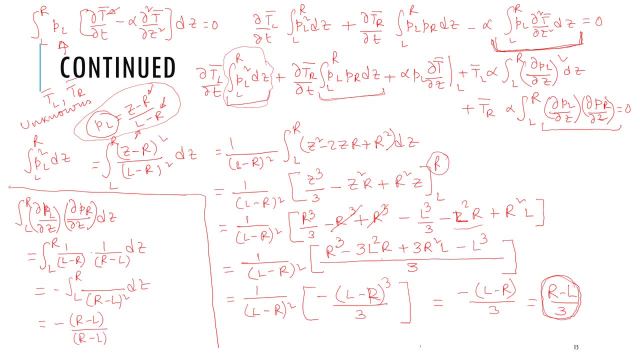 integrate R minus L square DZ, which is equal to minus R minus L, if we integrate out, and then R minus L square, which is minus 1 over R minus L. so now I hope you believe me that all of these terms can be integrated out, each one of them, okay. 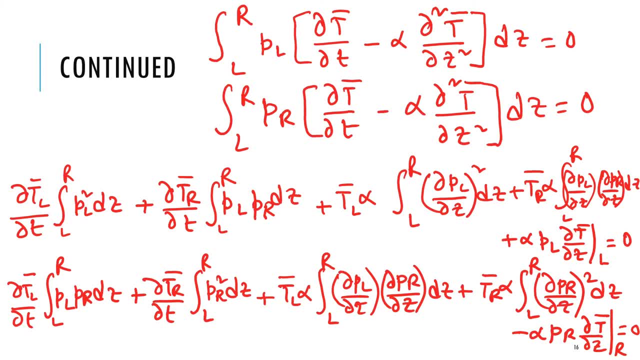 so the two equations that we got by doing weighted average equal to zero, those two equations we have been transforming one of them, so this is the first. this is the one that we were working on, and so, if we plugged in some of the changes that that we did, we have shown already that that one transforms. 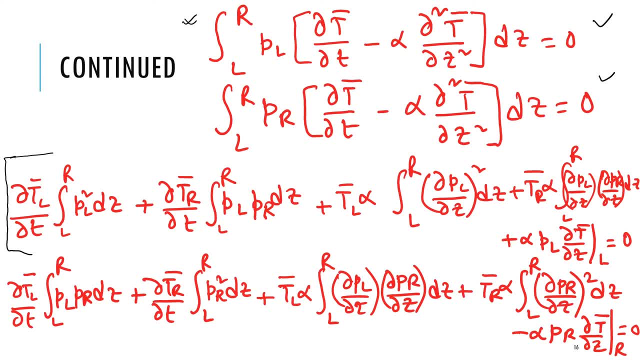 to this equation. we also have shown that these guys can be integrated out. I haven't done the integrate integration here. I put them in here to keep keep it general so far, but this equation became this one and then, if we go through the same process, then this second one is going to become this other. 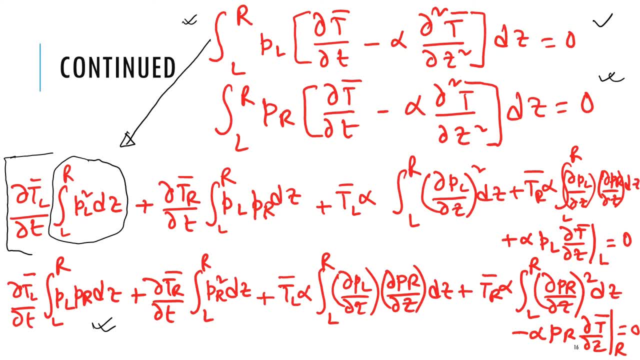 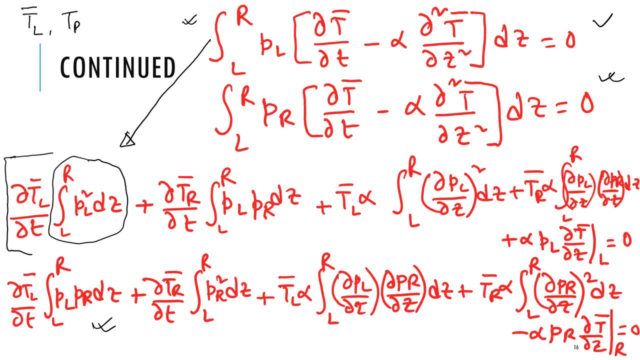 track of what we are after. we track of what we are after we want to solve for TL and TR. those are my want to solve for TL and TR. those are my want to solve for TL and TR. those are my unknowns. so two unknowns need two. 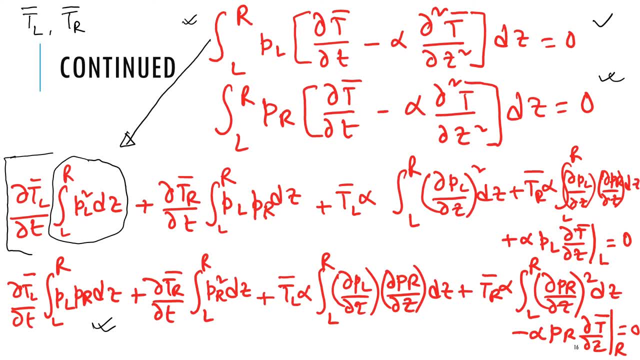 unknowns. so two unknowns need two unknowns. so two unknowns need two equations. we started from these from equations. we started from these from equations. we started from these from these guys, and then now we have these, these guys, and then now we have these, these guys, and then now we have these two, the two in the bottom, okay, and so in. 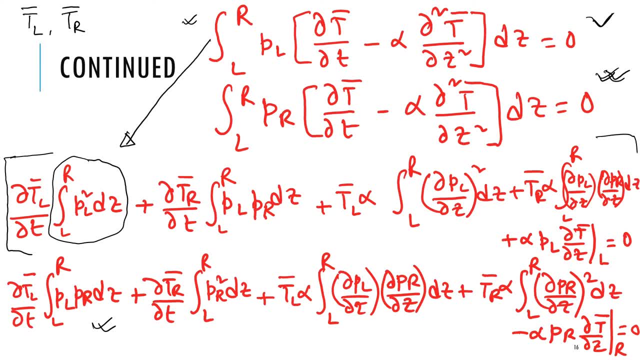 two, the two in the bottom, okay, and so in two, the two in the bottom, okay, and so in the next slide- we're going to simply the next slide- we're going to simply the next slide- we're going to simply write these two equations in. write these two equations in. 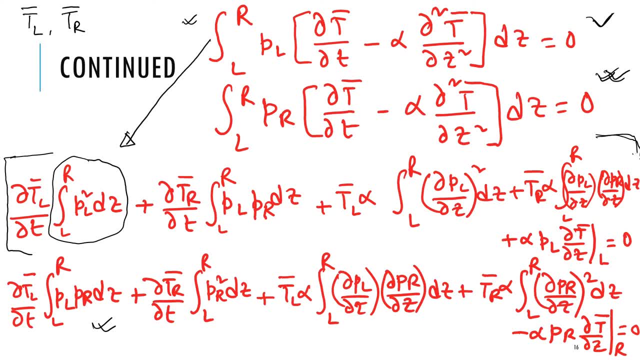 write these two equations in in a matrix form and we will hold off on in a matrix form and we will hold off on in a matrix form and we will hold off on actually integrating out of out these, actually integrating out of out these, actually integrating out of out these terms. but we know we can. so here we. 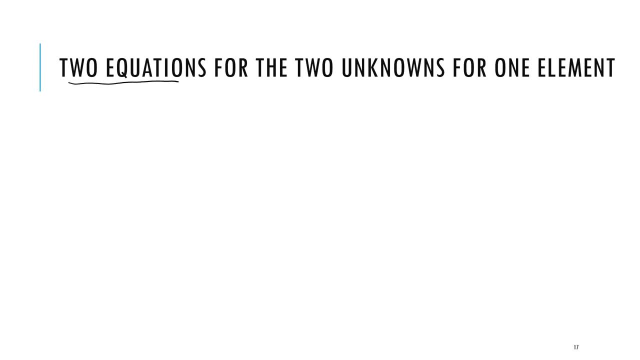 terms, but we know we can. so here we terms, but we know we can. so here we write those two equations for the two. write those two equations for the two. write those two equations for the two. unknowns in a matrix format here and unknowns in a matrix format here. and 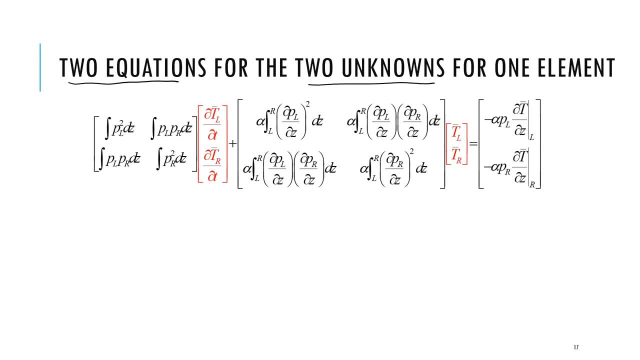 unknowns in a matrix format here, and those are the two equations that I just. those are the two equations that I just. those are the two equations that I just showed in the previous slide. and if, if we showed in the previous slide and if, if we showed in the previous slide and if, if we integrated out these, then it would 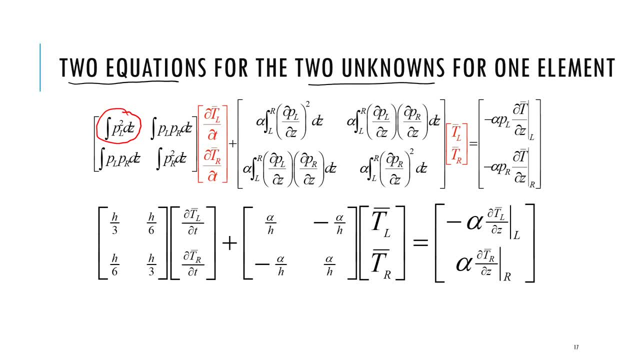 integrated out these, then it would integrated out these, then it would look: the two equations would would look like: look, the two equations would would look like: look, the two equations would would look like this: so you see, these things are this. so you see, these things are this. so you see, these things are known. this was my H, is my R minus L, this is: 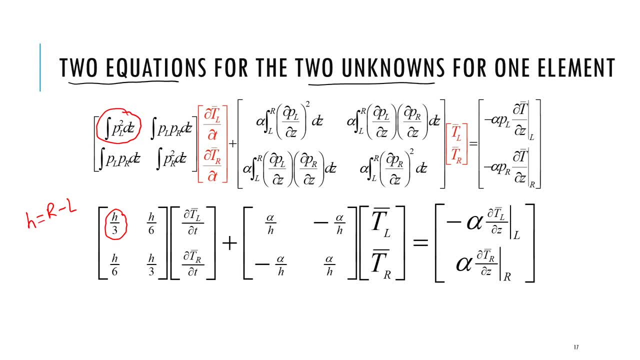 known. this was my H is my R minus L. this is known. this was my H is my R minus L. this is known. so this is how this is the known. so this is how this is the known. so this is how. this is the distance between the nodes that I choose. 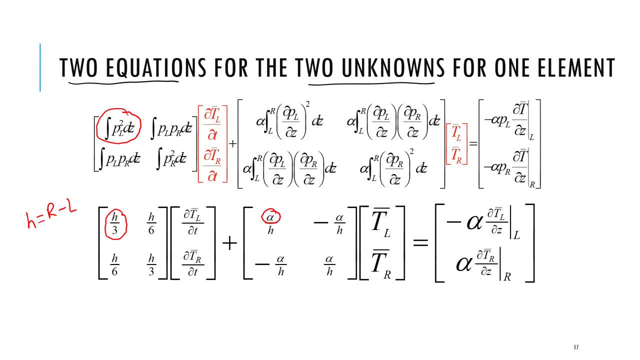 distance between the nodes that I choose, distance between the nodes that I choose, and in something like this and in something like this and in something like this, alpha is the thermal diffusivity, so alpha is the thermal diffusivity, so alpha is the thermal diffusivity. so that's a parameter that's given. so all 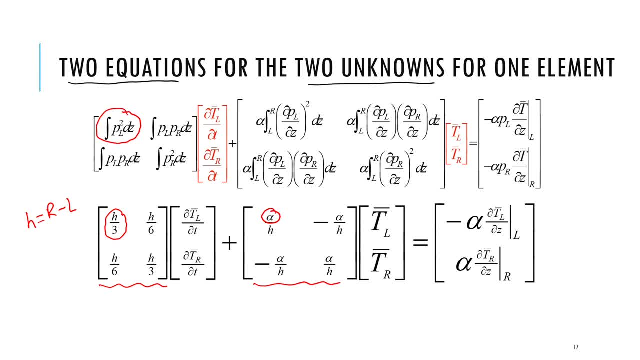 that's a parameter that's given. so all that's a parameter that's given. so all of this stuff is known okay. so we don't of this stuff is known okay. so we don't of this stuff is known okay. so we don't know these two that we will come back. 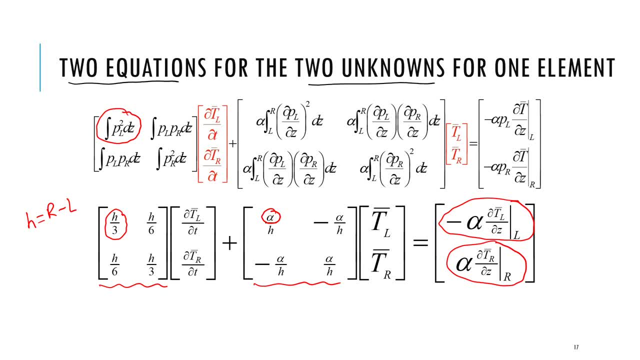 know these two that we will come back, know these two that we will come back very much, but this other stuff is known very much. but this other stuff is known very much, but this other stuff is known. so this is my two equations, so these are. so this is my two equations, so these are. 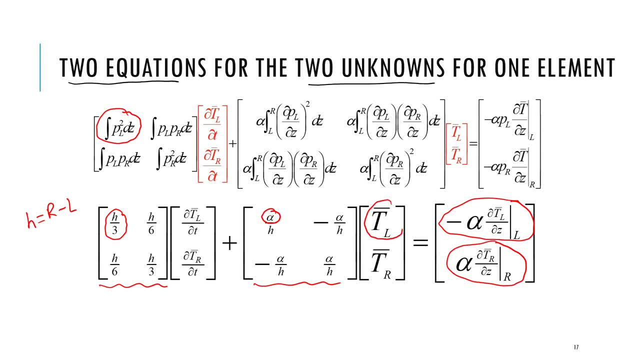 so this is my two equations. so these are my two equations for the two unknown, my two equations for the two unknown, my two equations for the two unknown: T, L and TR. okay. so two equations two: T L and TR. okay, so two equations two: T, L and TR. okay, so two equations, two unknowns for one element. and so I can. 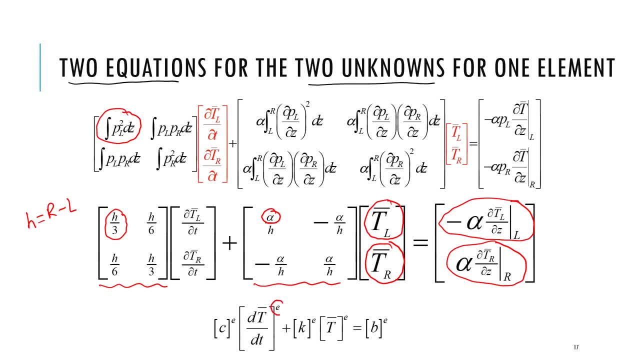 unknowns for one element, and so I can unknowns for one element, and so I can write it symbolically for that element. write it symbolically for that element. write it symbolically for that element. so e for element. so this DT, DT, so this, so this DT, DT, so this. 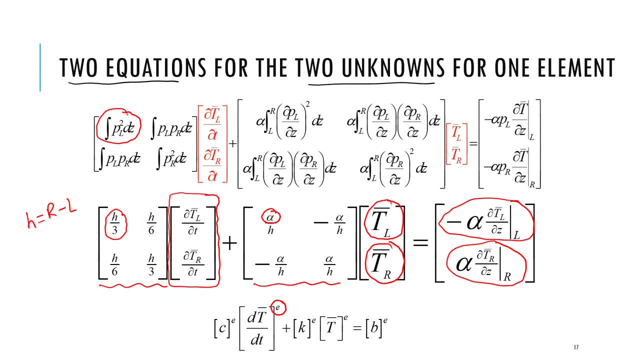 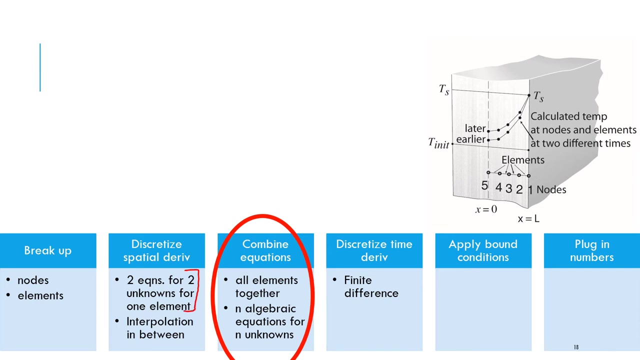 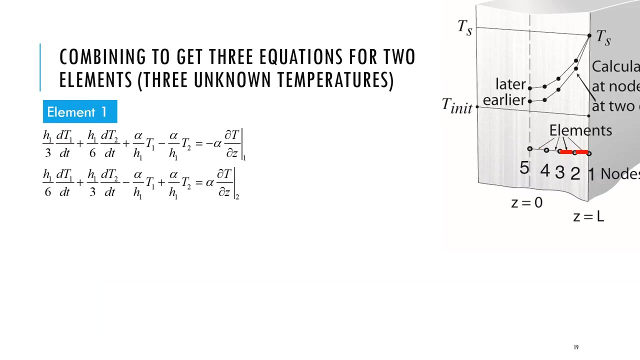 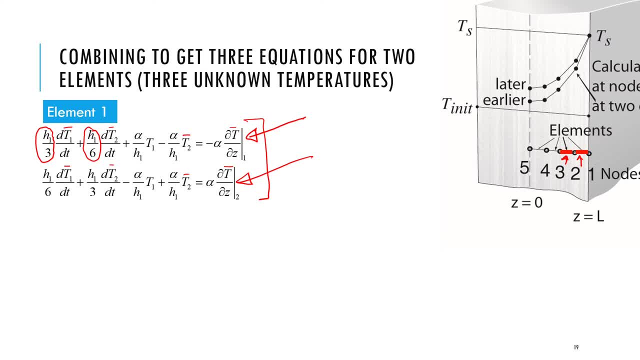 so, so you know, to solve for t1 and t2 bars we need two equations. we have two equations, but we have additional unknowns, so what to do about them. so let's write the equation also for the next element, that's element two. so this is element one. this is element two, so i write for element two. 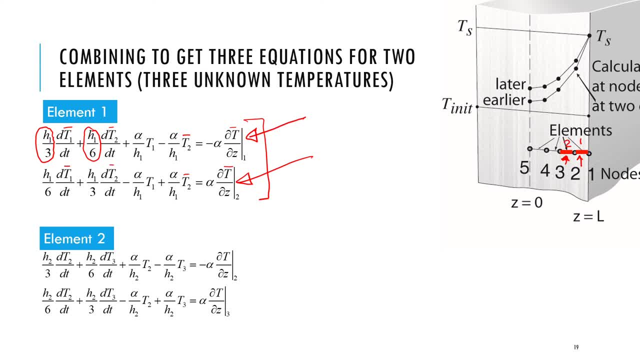 similar equation, very similar ones. so again you get two equations. now you notice that element two has this term that is same as in element one, but with an opposite sign. so now we can eliminate these by adding these two guys, meaning adding these two equations. but if we do that, then let's see what we get. 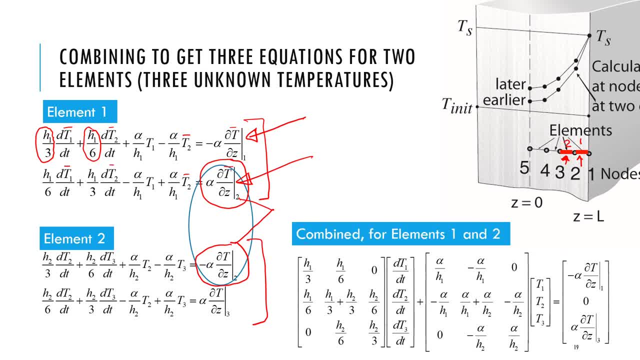 so if we combine the two, then we get this equation, where this the middle one, because those two are added, it's become 0 and these, since these two equations are added, we have only three equations: the first one, the second one which is: add, these two added. 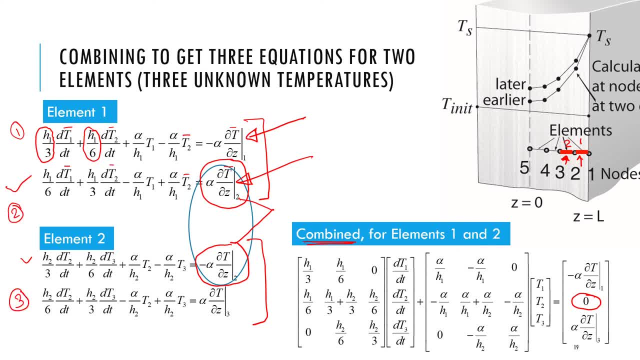 together and the third one, and that's what gives me this 3 by 3 matrix, with the three unknowns as t1 bar, t2 bar, t3 bar. they should all have bars in them, because they are my approximate result, and so then I no longer have these guys. 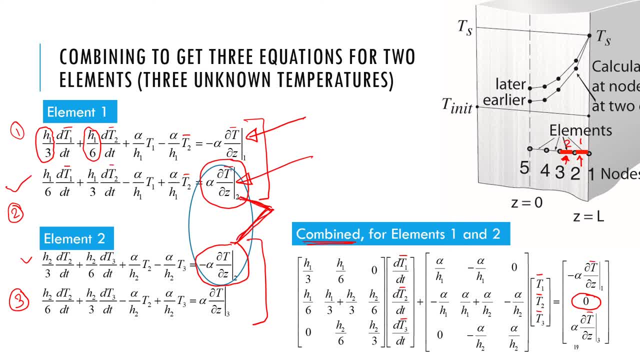 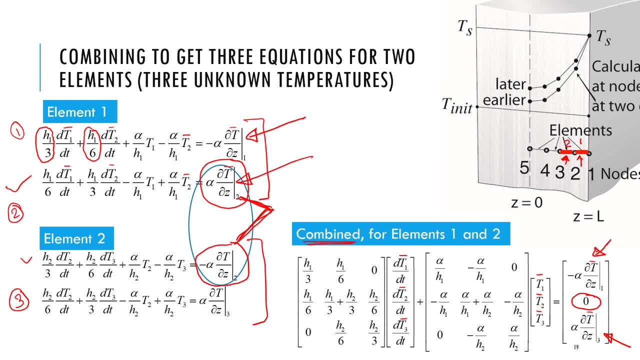 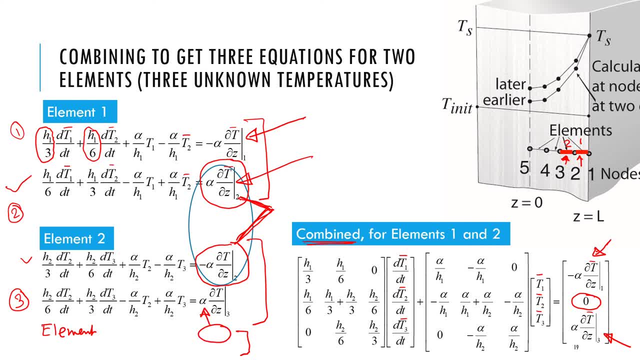 element 3. when we write the two equations, the first one would cancel out with this first one would cancel out with this first one would cancel out with this one. so all the middle ones will cancel out one. so all the middle ones will cancel out one. so all the middle ones will cancel out and we have the very last one. so if 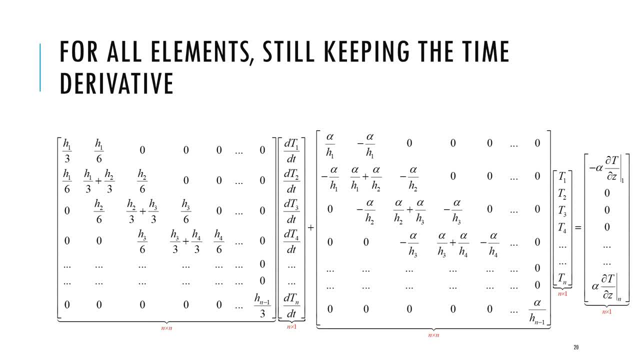 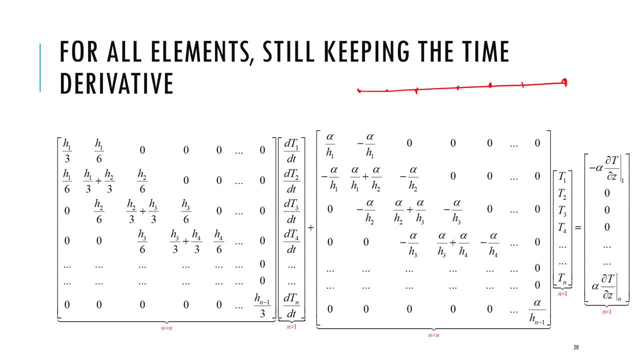 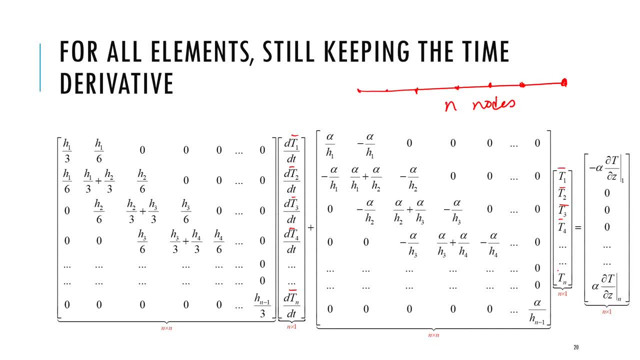 okay, so this t1, t2, t3, t4, t and these are okay. so this t1, t2, t3, t4, t and these are all the unknowns, so we have n unknowns, all the unknowns. so we have n unknowns, all the unknowns. so we have n unknowns, and so the number of elements would be n. 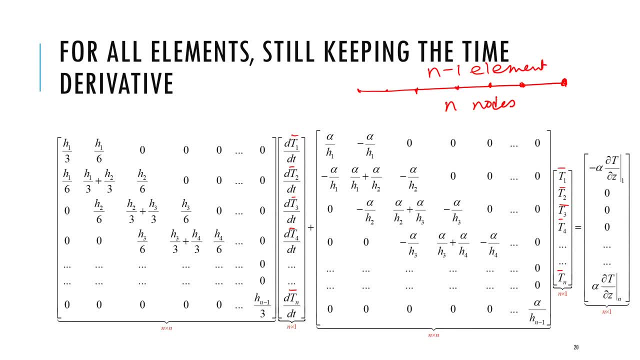 and so the number of elements would be n, and so the number of elements would be n minus 1 minus 1 minus 1 element. so if we divide the domain into n element, so if we divide the domain into n element, so if we divide the domain into n nodes, we get n minus 1 element. and so 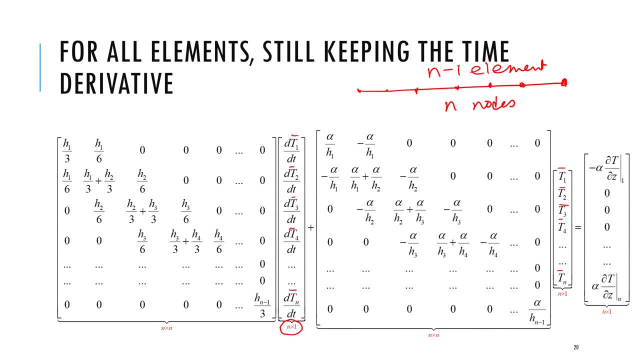 nodes: we get n minus 1 element, and so nodes, we get n minus 1 element. and so we have this matrix that is n by 1, so n. we have this matrix that is n by 1, so n. we have this matrix that is n by 1, so n. are those temperature values that we 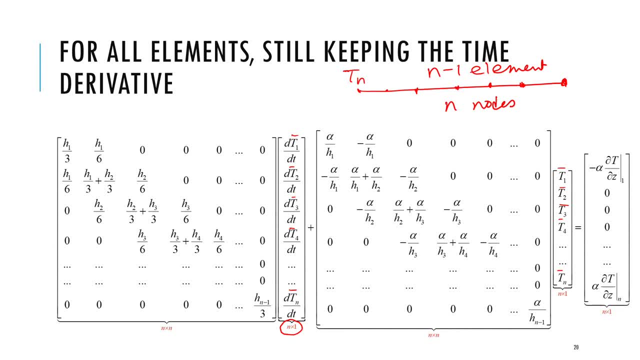 are those temperature values that we are those temperature values that we need to calculate. so T and T n minus 1 need to calculate. so T and T n minus 1 need to calculate. so T and T n minus 1, this is t1, t2. so those are the things we. 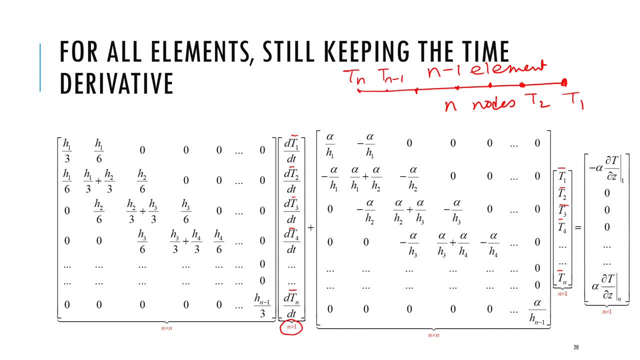 this is t1- t2. so those are the things we. this is t1- t2. so those are the things we need to calculate, and what I am showing need to calculate and what I am showing need to calculate, and what I am showing you here is simply the equation from the: 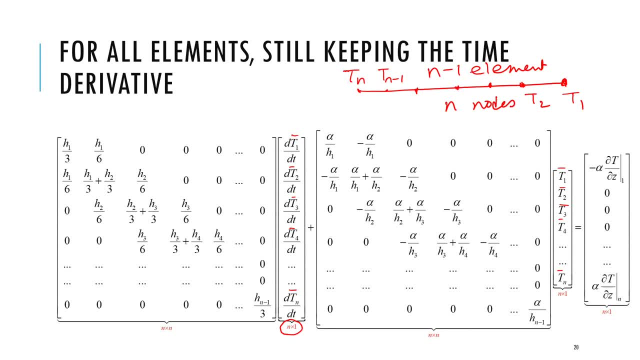 you. here is simply the equation from the. you here is simply the equation from the last slide, but expanded to more than two last slide, but expanded to more than two last slide, but expanded to more than two elements. okay, so now we get into elements. okay, so now we get into. 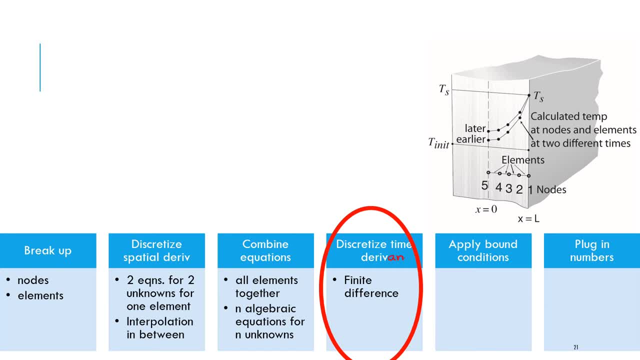 elements. okay, so now we get into discretizing the time derivative, discretizing the time derivative, discretizing the time derivative, derivative. and because you, you recall derivative, and because you, you recall derivative, and because you, you recall that you, we still have this kind of a, that you, we still have this kind of a. 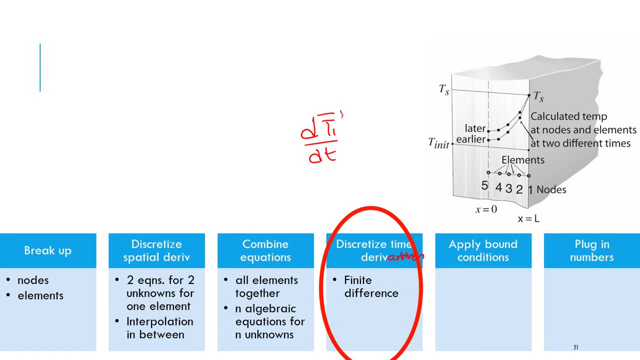 that you, we still have this kind of a term DT DT d1, term DT DT d1, term DT DT d1. okay, okay, okay, so the time derivative is still there. so, so the time derivative is still there. so so the time derivative is still there. so now we will discretize that. so back to 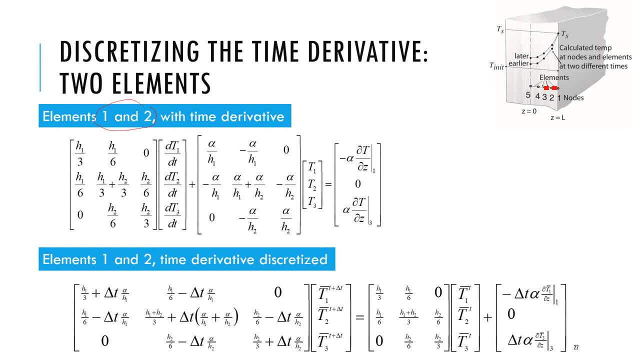 now. we will discretize that. so back to now, we will discretize that. so back to the equations for just two elements. the equations for just two elements. the equations for just two elements together. so two elements together there together. so two elements together, there together, so two elements together. there are three unknowns: t1, t2, t3, bars and and. 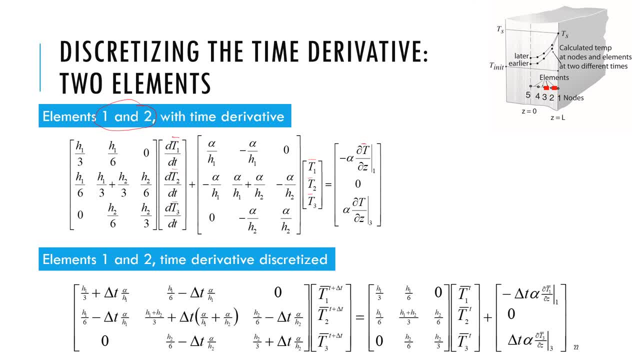 are three unknowns: t1, t2, t3 bars, and. and are three unknowns: t1, t2, t3 bars, and. and. so we have three equations now this. so we have three equations now this. so we have three equations now, this time derivative. we want to convert them, so I 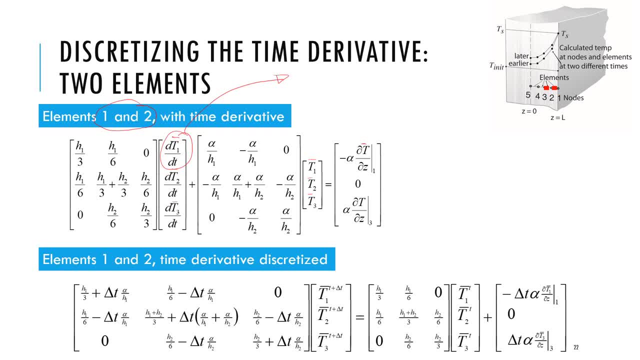 time derivative. we want to convert them, so I time derivative. we want to convert them so I can write the time derivative. can write the time derivative. can write the time derivative in in a very simple way, like like we do in. in in a very simple way, like like we do in. 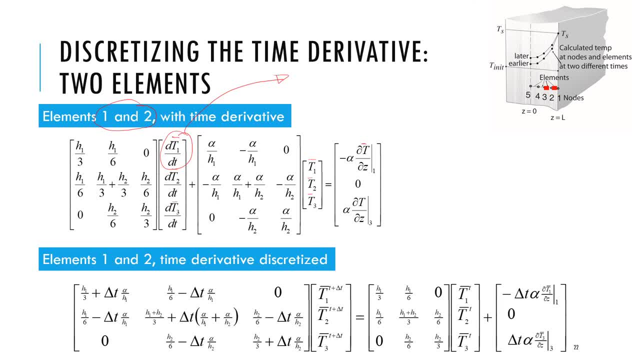 in in a very simple way, like like we do in finite difference, just for the time. finite difference, just for the time. finite difference just for the time derivative. so DT- this I can write as t1 derivative. so DT- this I can write as t1 derivative. so DT: this I can write as t1: t1 bar at T plus Delta T minus t1 at T. 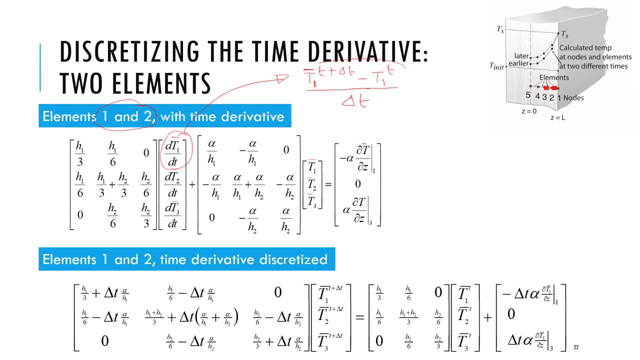 t1 bar at T plus Delta T, minus t1 at T. t1 bar at T plus Delta T, minus t1 at T over Delta T. so that's the you know over Delta T. so that's the you know over Delta T. so that's the you know, simple way of writing out. 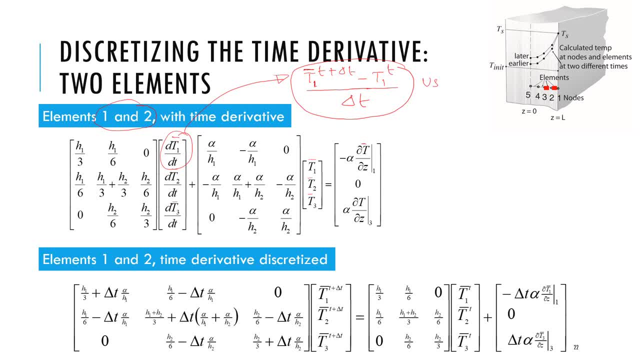 simple way of writing out, simple way of writing out: the time derivative in terms of values, the time derivative in terms of values. the time derivative in terms of values using finite difference. so this is also using finite difference. so this is also using finite difference. so this is also an approximation. okay, so if I write all 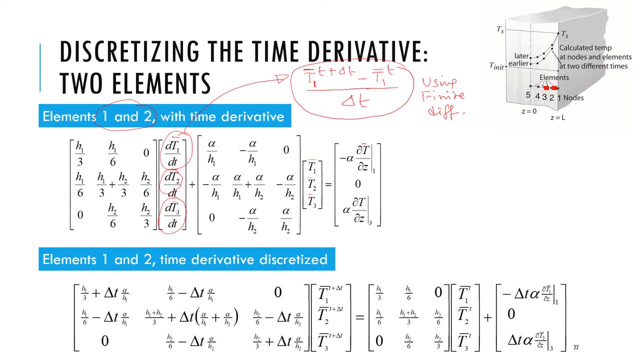 an approximation. okay. so if I write all an approximation, okay, so if I write all of the derivatives this way, and then of the derivatives this way, and then of the derivatives this way, and then simplify notice that we already have simplify notice that we already have simplify notice that we already have temperatures in there, okay, and so those. 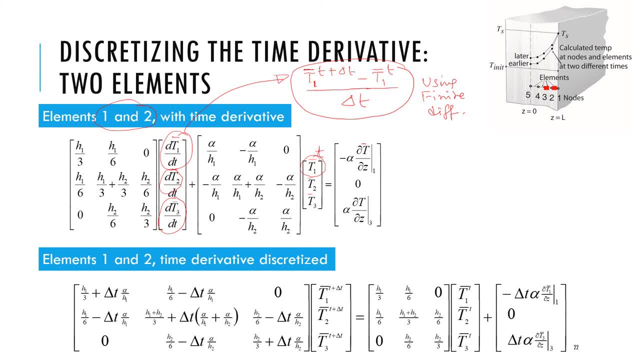 temperatures in there: okay, and so those temperatures in there, okay, and so those temperatures. let's say we temperatures. let's say we temperatures. let's say we assume them to be at time T, okay. so if assume them to be at time T, okay. so if assume them to be at time T, okay. so if we substitute these guys in there for 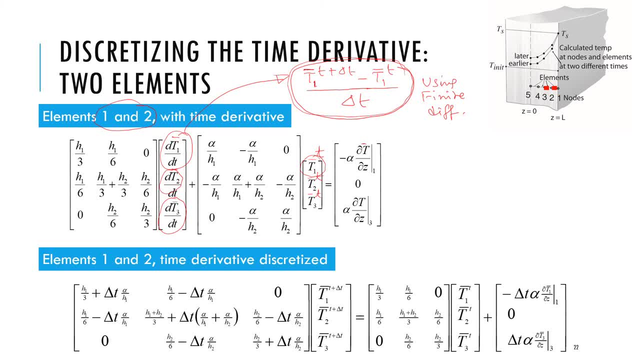 we substitute these guys in there, for we substitute these guys in there for derivatives, and then if we simplify derivatives, and then if we simplify derivatives, and then if we simplify again- and you can convince this yourself again, and you can convince this yourself again, and you can convince this yourself. but you can see clearly that if I 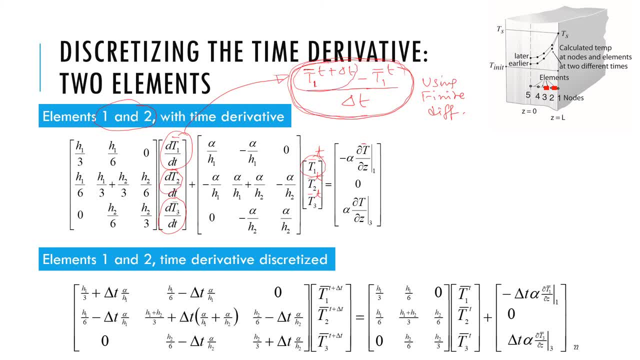 but you can see clearly that if I- but you can see clearly that if I substitute in here, then we would only substitute in here, then we would only substitute in here, then we would only have t1 at T plus Delta T and t1 at T, have t1 at T plus Delta T and t1 at T. 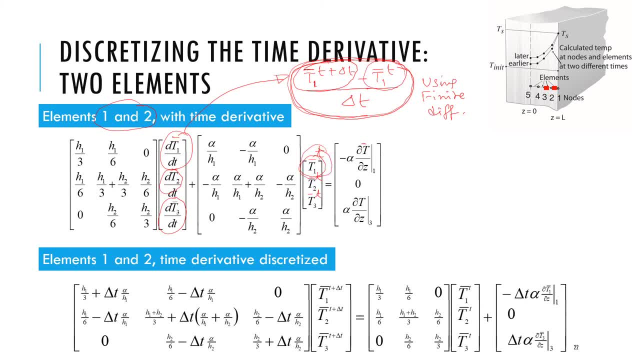 have t1 at T plus Delta T and t1 at T, then we collect all. then we collect all, then we collect all the terms that have t1 at T and, and then the terms that have t1 at T and, and then the terms that have t1 at T, and, and then we get this equation. so you notice what? 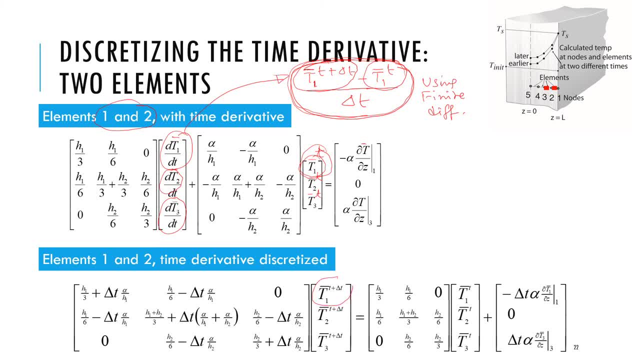 we get this equation so you notice what we get this equation so you notice what we have done. what is t1 at T plus Delta? we have done. what is t1 at T plus Delta? we have done. what is t1 at T plus Delta? T, that's the temperature at the next. 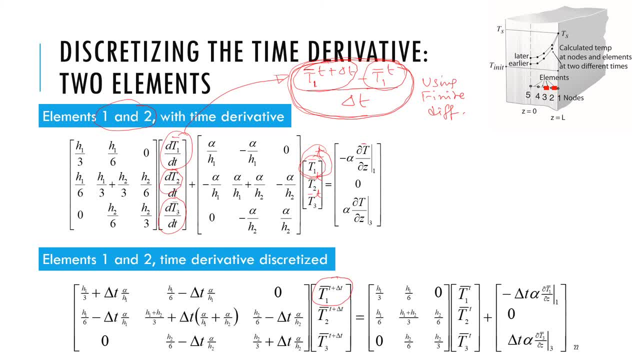 T, that's the temperature at the next T, that's the temperature at the next time step, and so that's on the right time step, and so that's on the right time step, and so that's on the right hand side. those are my unknowns to be. 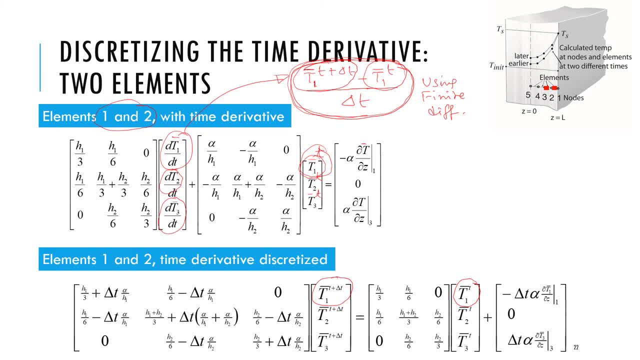 hand side, those are my unknowns to be hand side, those are my unknowns to be calculated. and on this side is t1 calculated and on this side is t1 calculated and on this side is t1 temperature at node 1 at time T, the 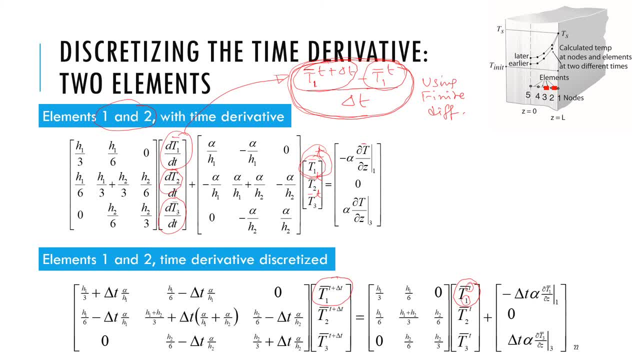 temperature at node 1 at time T. the temperature at node 1 at time T. the previous time step which we know, and previous time step which we know, and previous time step which we know and which we use to calculate the which we use to calculate the. 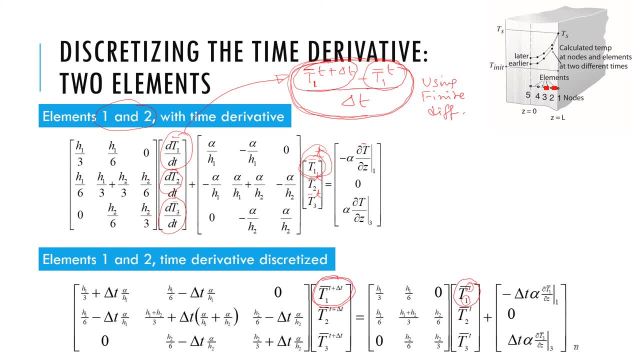 which we use to calculate the temperatures at time T plus Delta T and temperatures at time T plus Delta T and temperatures at time T plus Delta T. and we can march on this way. so you notice, we can march on this way. so you notice, we can march on this way. so you notice, something really big has happened, so we 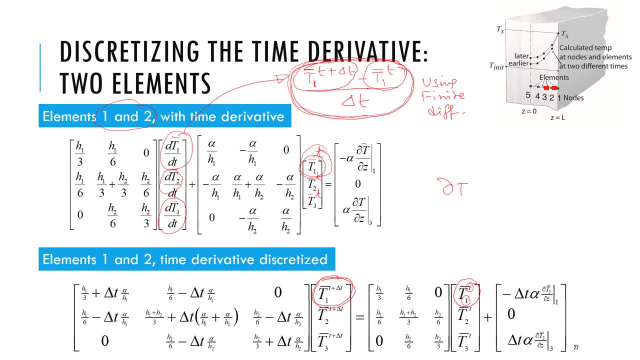 something really big has happened, so we something really big has happened, so we started off with the heat equation del, started off with the heat equation del, started off with the heat equation del: T del T alpha del square, T del Z square, T del T del T alpha del square, T del Z square. 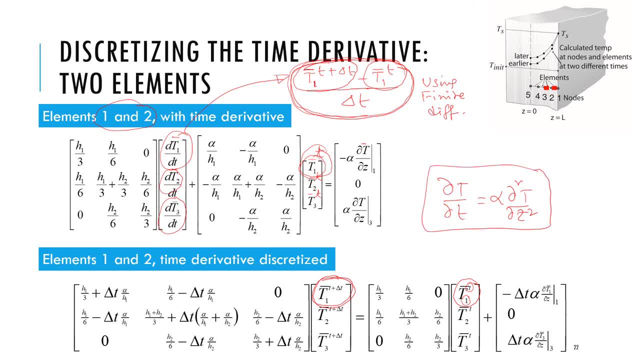 T del T del T, alpha del square, T del Z square. we didn't go through the series. we didn't go through the series. we didn't go through the series solution or some other analytical solution solution or some other analytical solution solution or some other analytical solution procedure, but we converted them. 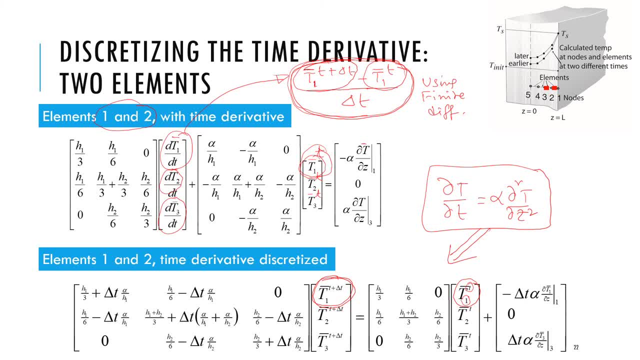 procedure, but we converted them. procedure, but we converted them like we wanted to. we converted them into like we wanted to. we converted them into like we wanted to. we converted them into algebraic equations. so these are just algebraic equations. so these are just algebraic equations. so these are just algebraic equations, all these things are. 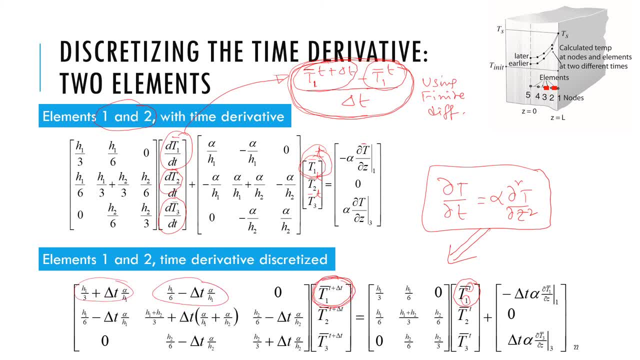 algebraic equations. all these things are algebraic equations. all these things are known. so we can always solve for t1 at T known. so we can always solve for t1 at T known. so we can always solve for t1 at T plus Delta T, because everything on the 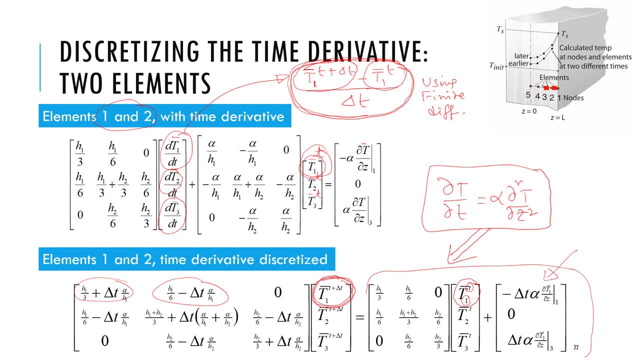 plus Delta T, because everything on the plus Delta T, because everything on the right-hand side is also known without right-hand side is also known without right-hand side, is also known without these guys. we will show you that these, these guys, we will show you that these 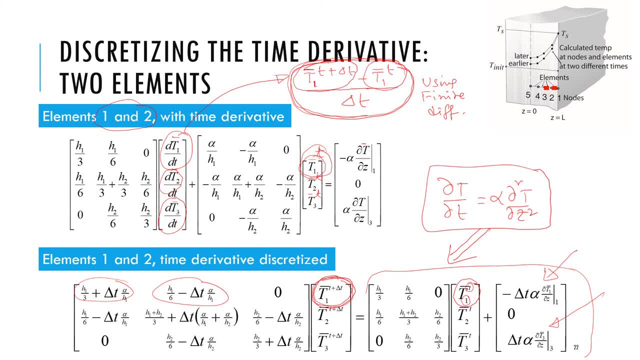 these guys. we will show you that these also can be found. but for now, assume also can be found. but for now, assume also can be found. but for now assume they can also be found. so everything on, they can also be found. so everything on they can also be found. so everything on the right-hand side is known. so this is. 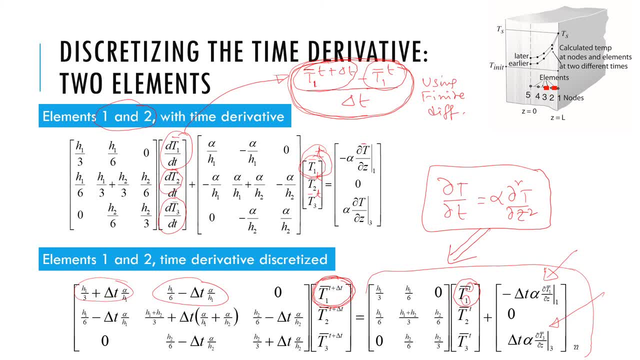 the right-hand side is known. so this is the right-hand side is known. so this is a big deal that we converted a. a big deal that we converted a a big deal that we converted a differential equation into just algebraic, differential equation into just algebraic. 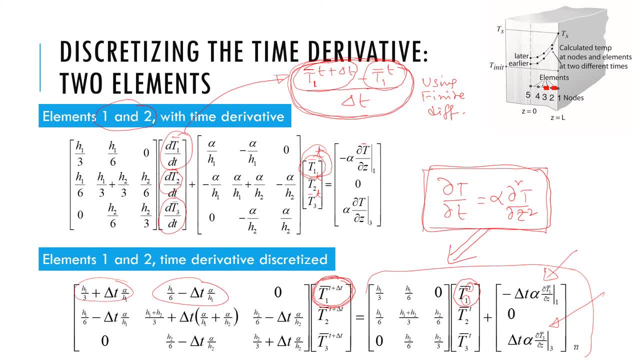 differential equation into just algebraic equation now, instead of just playing equation now, instead of just playing equation now, instead of just playing with these two element equations, just with these two element equations. just with these two element equations, just one and two. we will go back to the more. 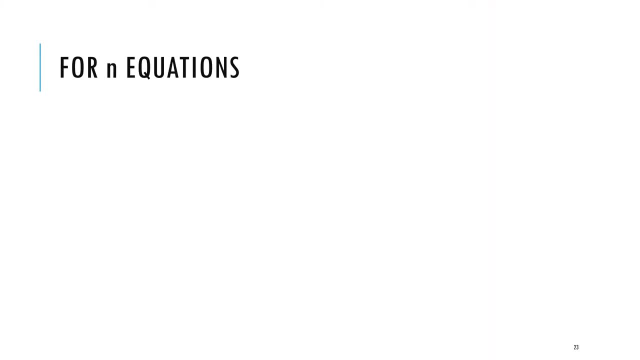 one and two. we will go back to the more one and two. we will go back to the more general one with all the elements. so the general one with all the elements, so the general one with all the elements, so the one with all the elements in there. that 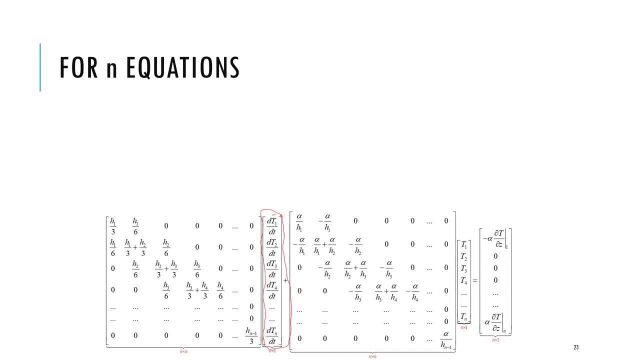 one with all the elements in there, that one with all the elements in there that I had showed earlier. looks like this I had showed earlier. looks like this I had showed earlier. looks like this, with with all the elements in there and with with all the elements in there, and. 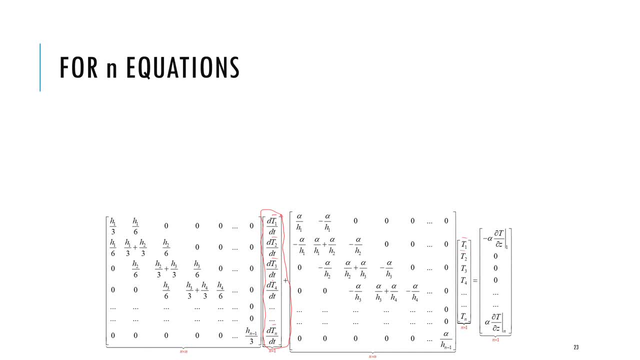 with with all the elements in there, and and they should all be the approximate and they should all be the approximate and they should all be the approximate. values okay, values, okay, values, okay, okay, values, okay, okay. so I can write this entire matrix now. so I can write this entire matrix now. 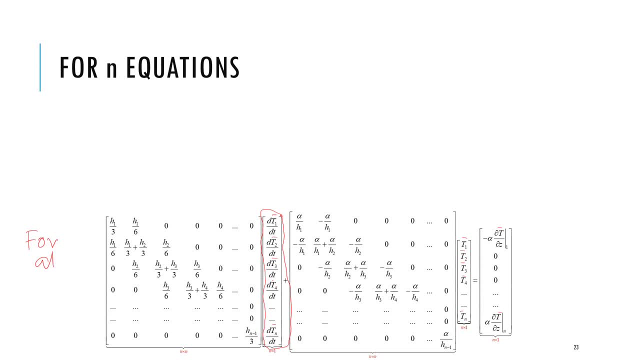 so I can write this entire matrix now. so this is for all elements together, for so this is for all elements together, for so this is for all elements together, for all elements together, okay. so that's why all elements together, okay. so that's why all elements together, okay. so that's why it it has n equations for n unknowns, n. 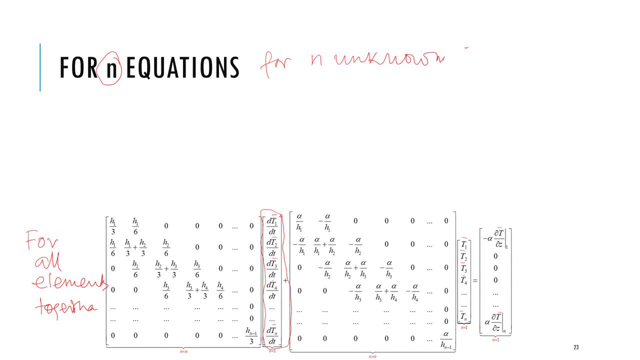 it. it has n equations for n unknowns n it. it has n equations for n unknowns: n unknowns: t1 bar, t2 bar, and so on. T n bar unknowns. t1 bar, t2 bar, and so on. T n bar unknowns. t1 bar, t2 bar, and so on. T n bar okay. 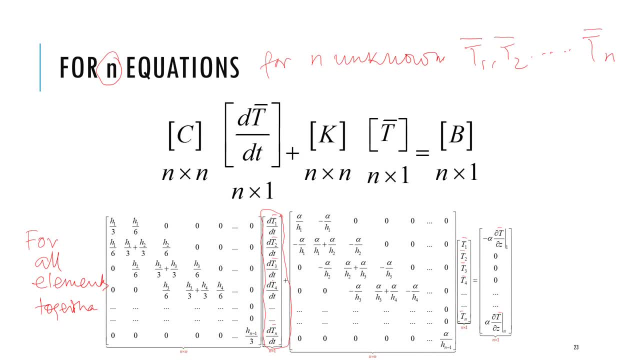 okay, okay, okay. so if I write this in symbolic form, then so if I write this in symbolic form, then so if I write this in symbolic form, then this I call the C matrix and this is the. this I call the C matrix and this is the. this I call the C matrix and this is the DT DT matrix. so this would be n by 1. 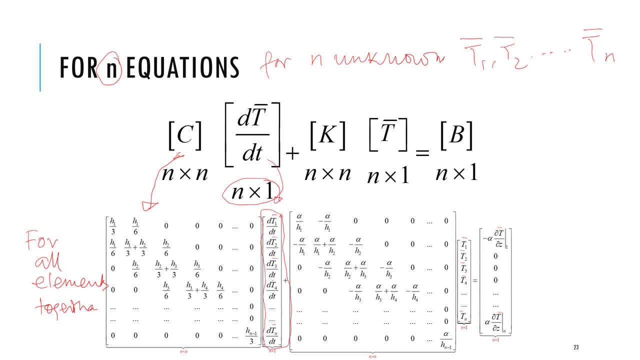 DT- DT matrix. so this would be n by 1. DT- DT matrix. so this would be n by 1. because we have n unknowns and, and so because we have n unknowns and, and so because we have n unknowns, and, and so then this matrix would be n by n and. 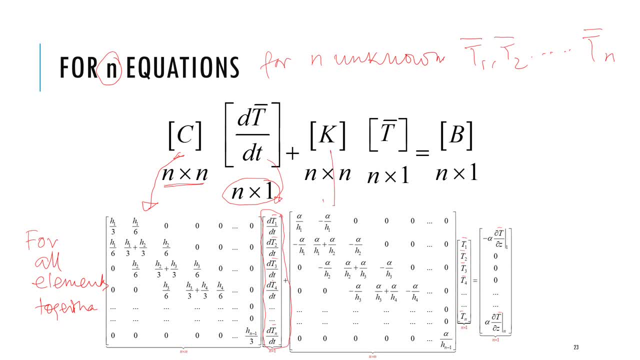 then this matrix would be n by n, and then this matrix would be n by n, and then, likewise, this is my K matrix. and then likewise, this is my K matrix. and then, likewise, this is my K matrix, and then, of course, T matrix is again. then, of course, T matrix is again. 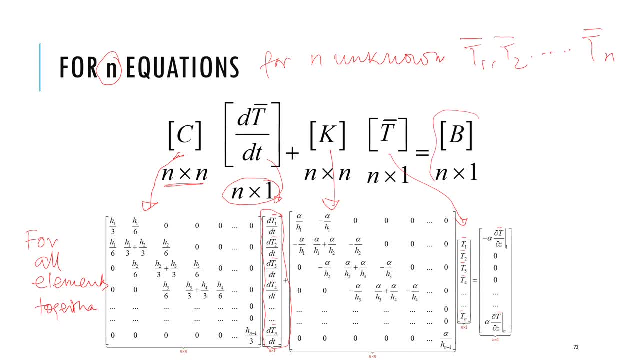 then of course T matrix is again n by 1, and so the right hand side would n by 1, and so the right hand side would n by 1, and so the right hand side would of course have to be the same n by 1. so 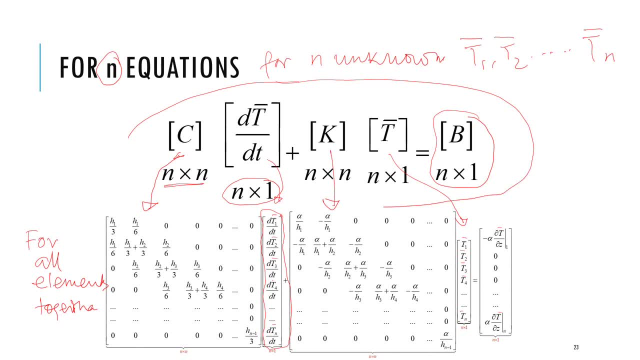 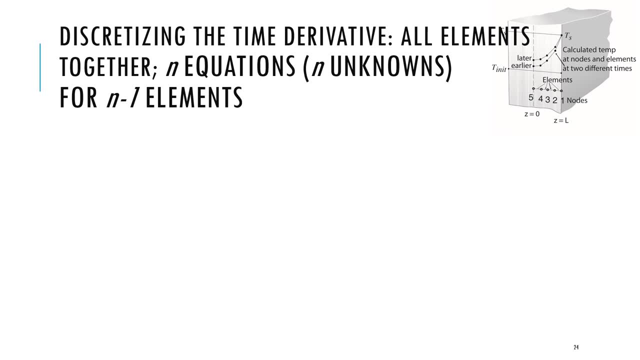 of course have to be the same- n by 1. so of course have to be the same n by 1. so this is my equation for the entire. this is my equation for the entire. this is my equation for the entire system. okay, we now go back to the full. 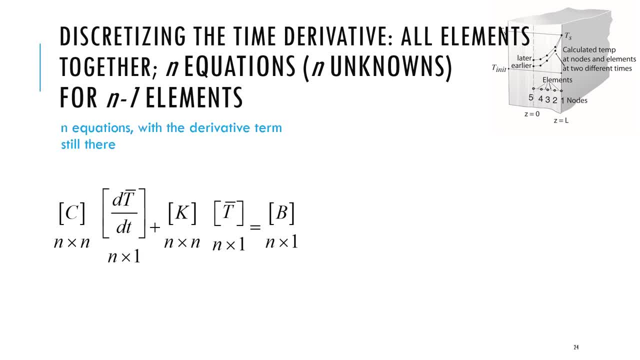 system. okay, we now go back to the full system. okay, we now go back to the full system of equations to change the time system of equations, to change the time system of equations, to change the time derivative. so this is the full set of derivative. so this is the full set of. 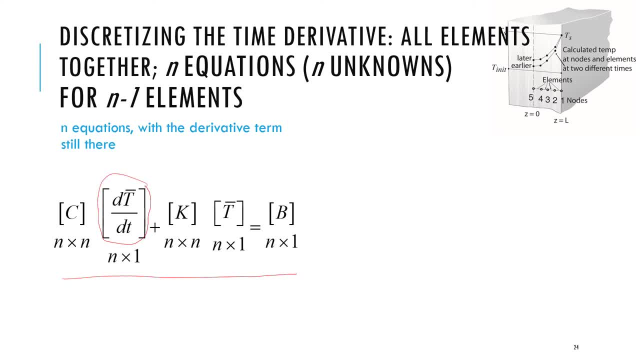 derivative. so this is the full set of equations and it still has the time equations and it still has the time equations and it still has the time derivative in there which we now want to derivative in there which we now want to derivative in there which we now want to change. now there can be many ways of 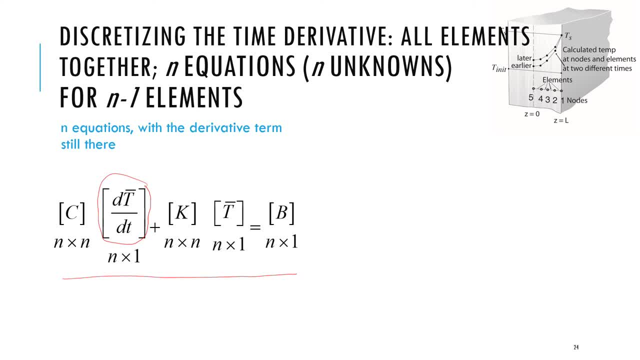 change. now there can be many ways of change. now there can be many ways of writing the derivative one. we already writing the derivative one. we already writing the derivative one. we already tried a few minutes ago. the two common tried a few minutes ago. the two common tried a few minutes ago. the two common choice for discretization is one can be. 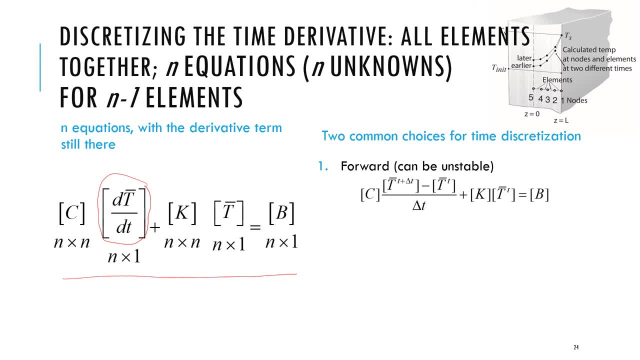 choice for discretization is one can be. choice for discretization is one can be forward. this is the one that I just did forward. this is the one that I just did forward. this is the one that I just did a few minutes ago. so the forward one DT. 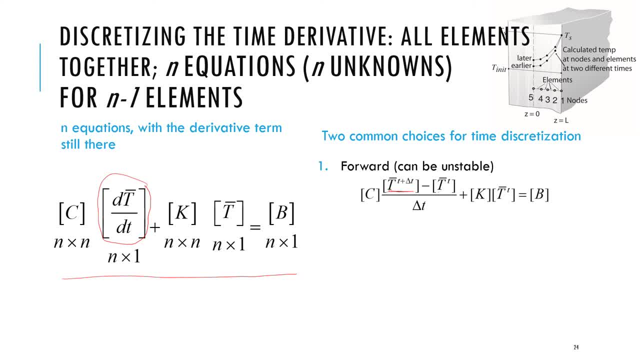 a few minutes ago, so the forward one DT a few minutes ago, so the forward one. DT. DT is simply T at T plus Delta T minus T. DT. DT is simply T at T plus Delta T minus T. DT. DT is simply T at T plus Delta T minus T at T over Delta T and these. 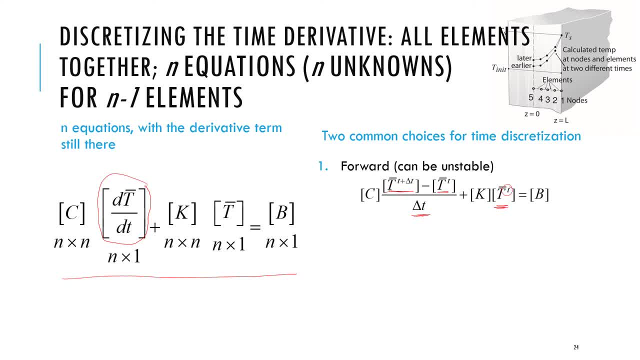 at T over Delta T and these at T over Delta T, and these temperatures are taken at the current temperatures, are taken at the current temperatures, are taken at the current time step and from there, if I do the time step and from there if I do the time step and from there if I do the algebra, then I collect all the terms. 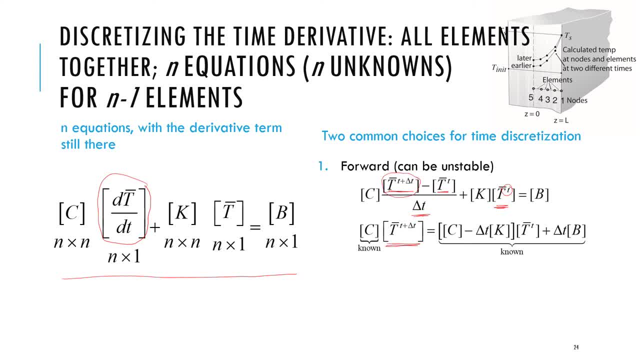 algebra, then I collect all the terms algebra. then I collect all the terms related to T plus Delta T on this side, related to T plus Delta T on this side, related to T plus Delta T on this side, and all the terms related to and all the terms related to. 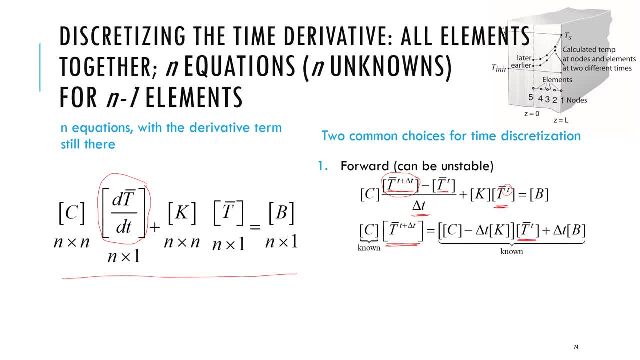 and all the terms related to temperature, temperature. temperature is at T on this side, and so you notice, is at T on this side, and so you notice, is at T on this side, and so you notice. now, this is a set of algebraic equations. now, this is a set of algebraic equations. 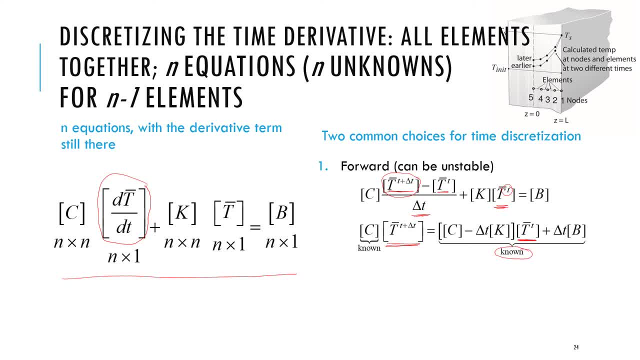 now, this is a set of algebraic equations where everything is known on the right, where everything is known on the right, where everything is known on the right hand side, and we are solving for these hand side, and we are solving for these hand side and we are solving for these temperatures at our next time step. 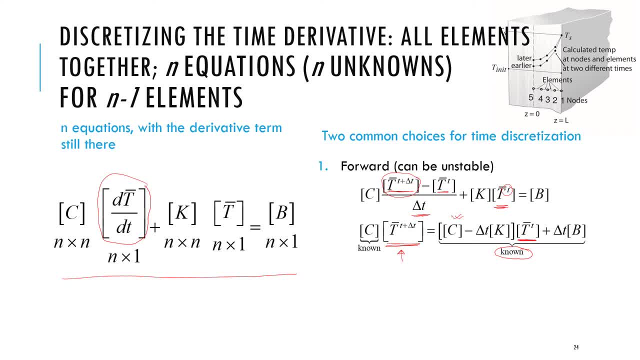 temperatures at our next time step. temperatures at our next time step. everything is known because, as I already, everything is known because, as I already, everything is known because, as I already discussed these quantities inside the, discussed these quantities inside the, discussed these quantities inside the matrix. they are known because we know. 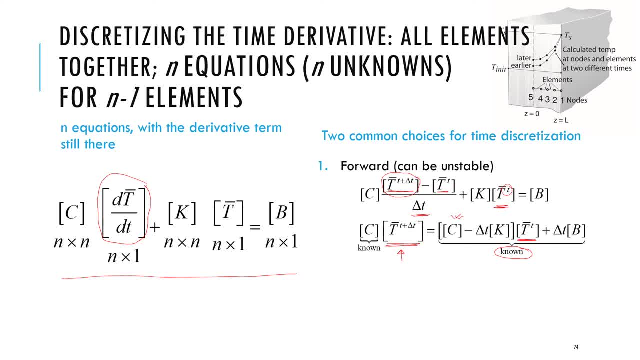 matrix. they are known because we know matrix. they are known because we know what, what, what and the size- the element size we chose. and the size- the element size we chose. and the size, the element size we chose. and so on. likewise, we know what is the, and so on. likewise, we know what is the. 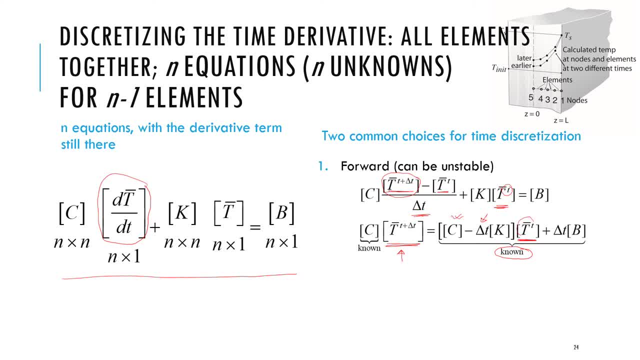 and so on. likewise, we know what is the time step and so, and then we also know time step and so, and then we also know time step and so, and then we also know the temperatures at the current time, the temperatures at the current time, the temperatures at the current time step. so from there we can find. 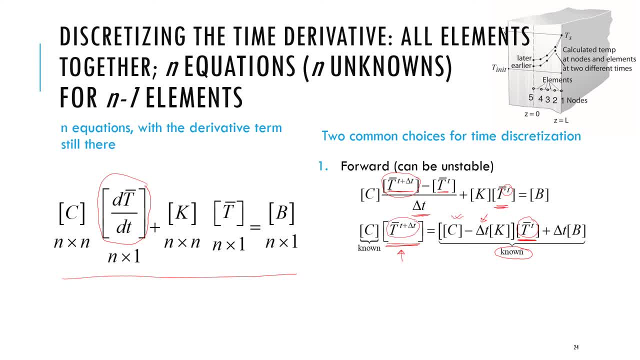 step, so from there we can find step. so from there we can find temperature at the next time, step. so temperature at the next time, step, so temperature at the next time, step. so this is a set of algebraic equations. this is a set of algebraic equations. 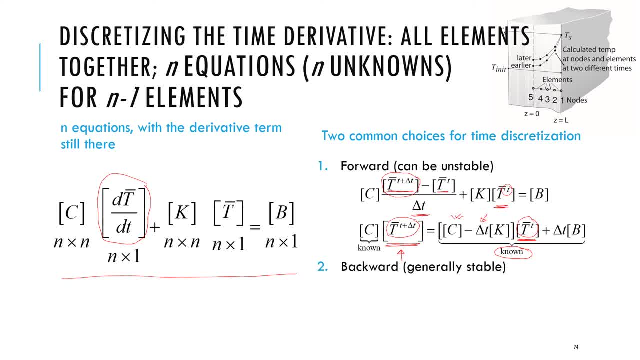 this is a set of algebraic equations, like I showed in the matrix form before, like I showed in the matrix form before, like I showed in the matrix form before, the other choice of changing the time, the other choice of changing the time, the other choice of changing the time, derivative is, is, is this way, where this 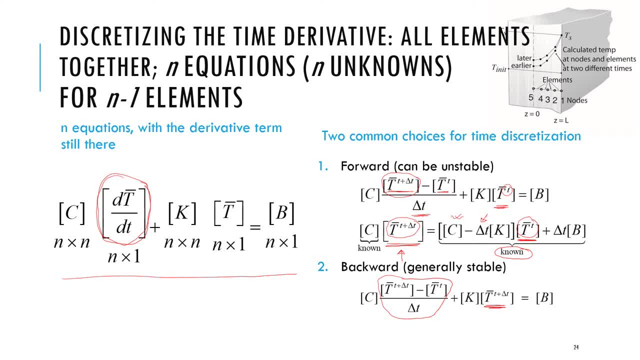 derivative is. is this way where this derivative is? is this way where this? this temperature here is taken at the. this temperature here is taken at the. this temperature here is taken at the time step to be calculated. that makes it time step to be calculated. that makes it. 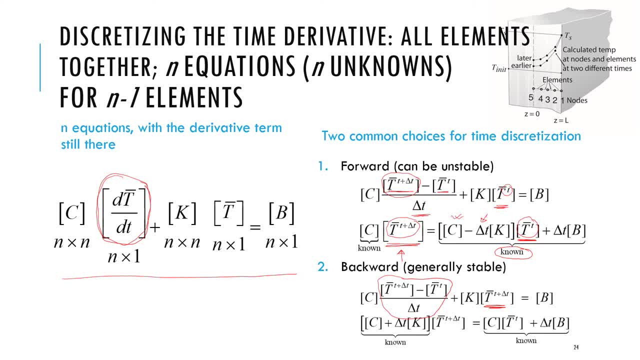 time step to be calculated. that makes it implicit, that makes it a bit different. implicit, that makes it a bit different. implicit, that makes it a bit different. so again, if we collect all the terms, so again, if we collect all the terms, so again, if we collect all the terms together, 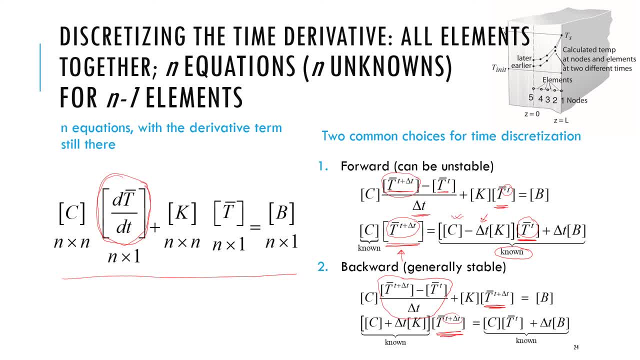 together for temperatures at t plus delta t and temperatures at t, then the final equation looks like this: this is a bit different from here, but the calculation behavior for them can be quite different. so whereas this one can often can become unstable, this one is typically quite stable in calculations, meaning it will not give. 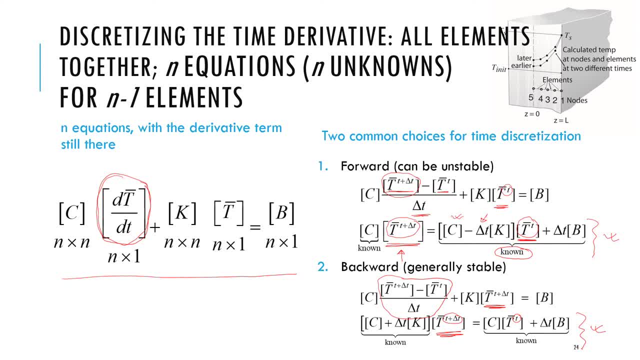 garbage that easily. we can take larger time step, so these details we're not getting into. i would like you to see that the derivative, the time derivative, has been transformed or can be transformed in one of two ways. after that it is nothing but a time step. so this one is typically quite stable in calculations, meaning it will not. 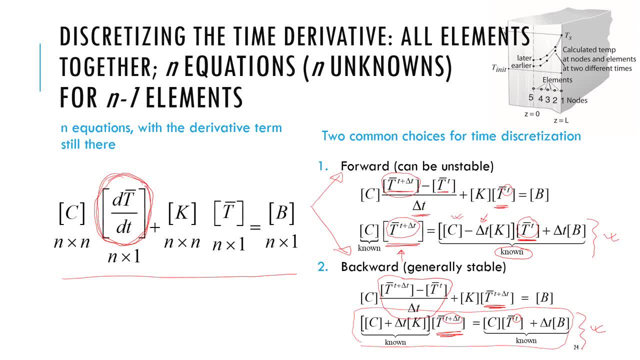 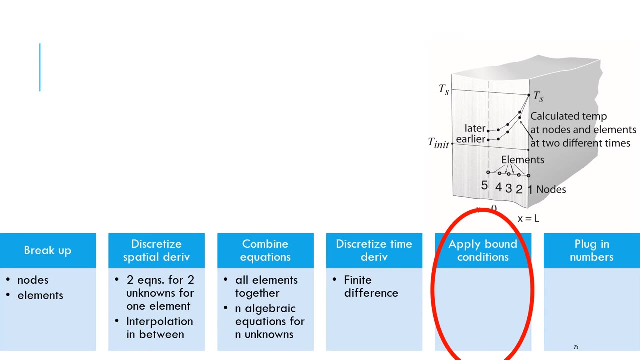 give anything but an algebraic equation. so then in here, our heat equation has been completely converted into an algebraic equation, so we just now need to solve a set of linear equation, simultaneous linear equations, now that we have a set of algebraic equations. so we have converted everything from. 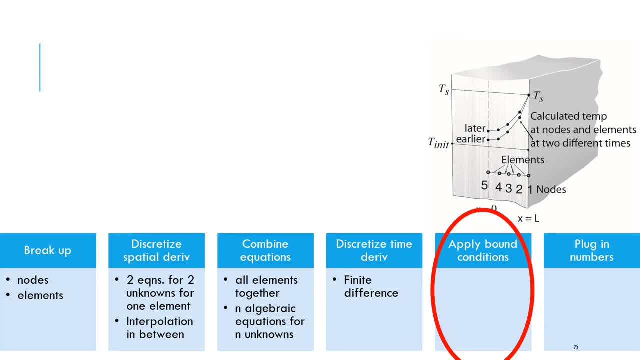 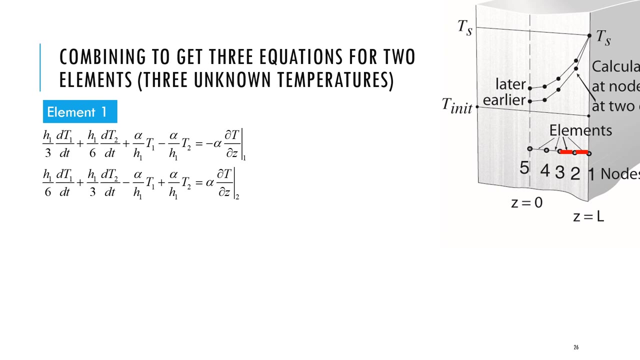 a, the spatial derivative and the time derivative- to a set of algebraic equations. we just need to apply the boundary conditions, which we haven't done so far. so just to recap, when we wrote the two equations for element one- that's this, and then element one- i mean two, this- then we combined these two and we eliminated these two terms. 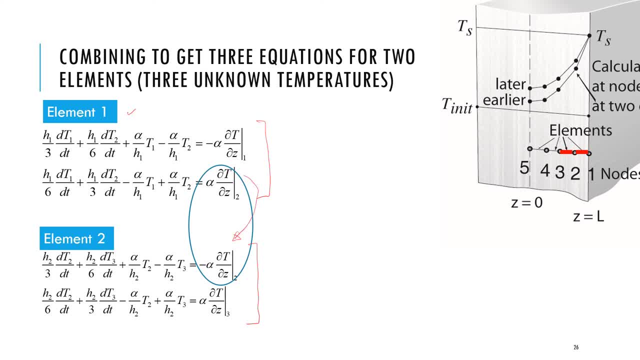 this one and this one got together when we added they got eliminated. so we showed that all of these middle or the interior terms can be eliminated, but the first one and the last one, last one, are going to stay. so these are still unknowns, unknown and unknown here. 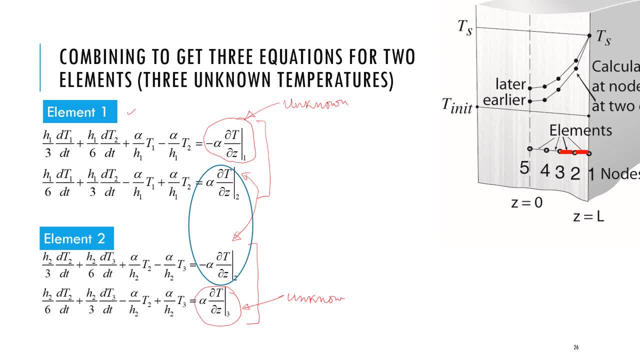 okay. so these are also. you notice, they're at node one and they're at node three, in this case for two elements. so it's this end. so if we do this for all the elements, then the the last one is going to be node five. so those are the boundaries. 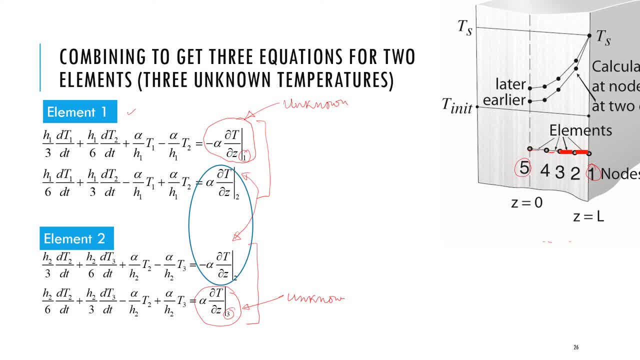 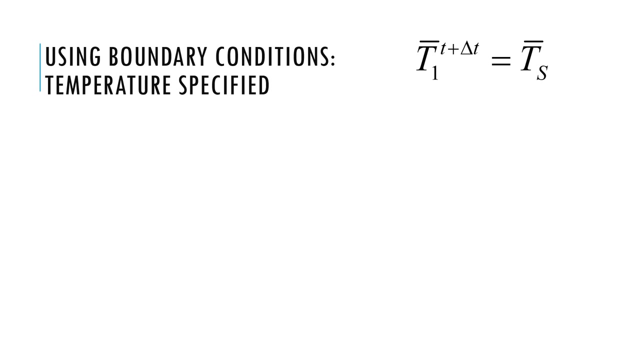 and so, coincidentally, we have not even used boundary conditions so far. so we will use the two boundary conditions here and here to evaluate these two guys, okay, so so those are the ones that we need the boundary conditions for, for this two-noded element. so we're going to go through three common types of boundary conditions. one is temperature. 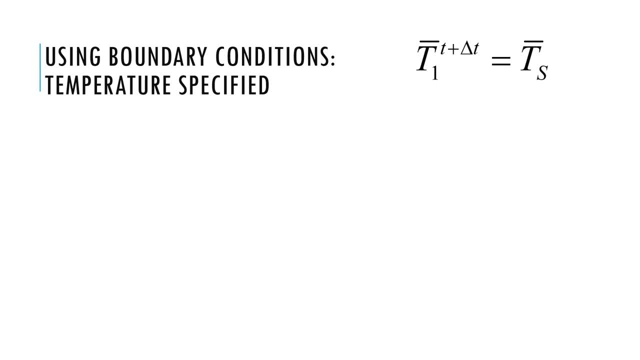 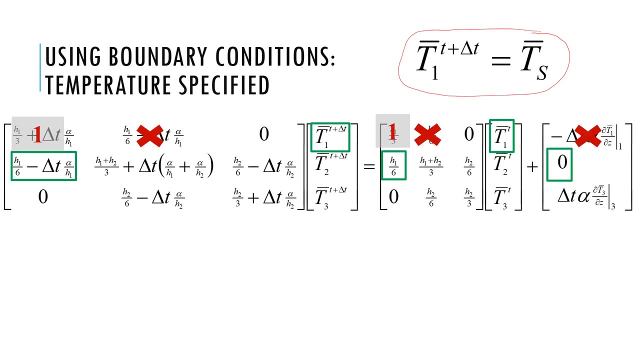 specified, the other is heat flux and the last one is convection, as you have seen in a heat transfer class. so the first one is this: temperature specified. so for temperature specified boundary condition, you notice that the equation that we have now, this is of course, for the 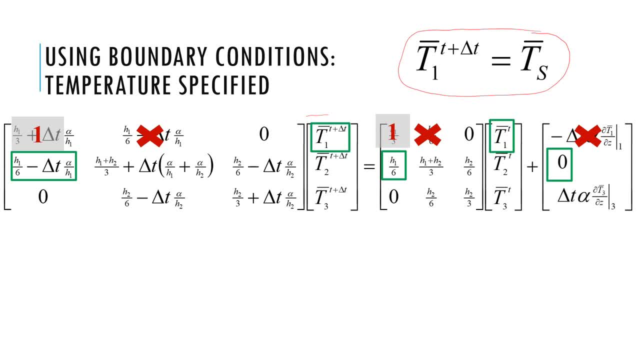 two-noded element. so these are the temperatures we are going to solve for. these are the unknowns. but notice, if this boundary temperature is given as it is here, then this is not something we need to solve for. so then the way this is implemented is: is we force? 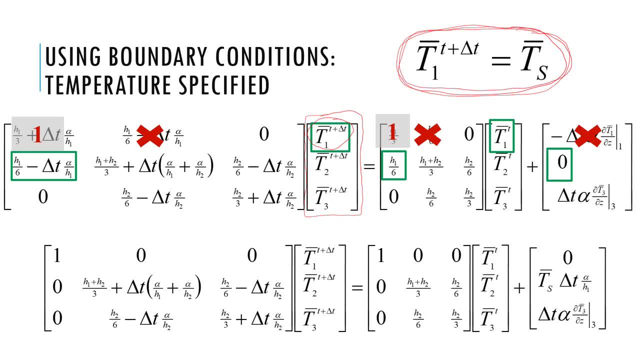 this condition as one of the equations, so we replace the first equation by this one. so this basically says that t1, t is equal to t, s or the temperature at the previous time step at one, which is a known condition. okay, so this boundary condition is handled this way. 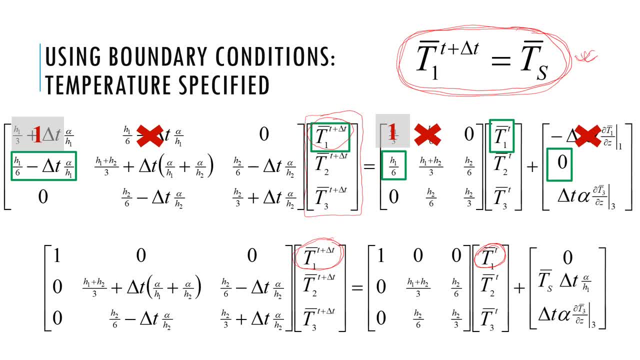 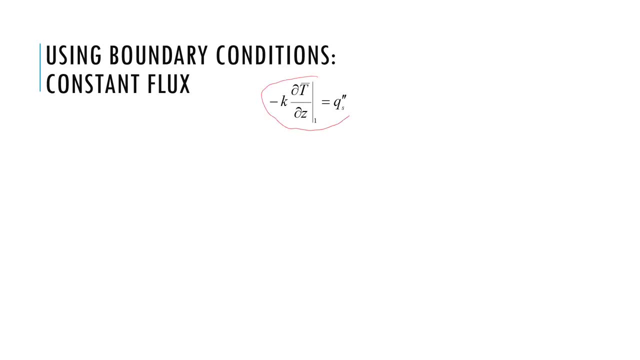 because this basically says that the, the for the boundary, the temperature is already known, so you wouldn't be solving for it. so this is how it's handled. the next one is flux specified. so you remember, flux specified boundary condition is written this way: so this is: the conductive flux is equal to the flux value given at the. 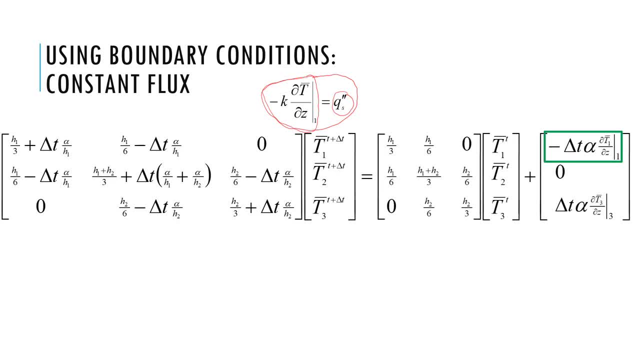 boundary. now you notice interestingly in our equation, the, the term, already needs this gradient. it needs the gradient, so this works out very conveniently. so all we need to do is from this: we replace, you know, del t. del z is equal to minus q, s over k. 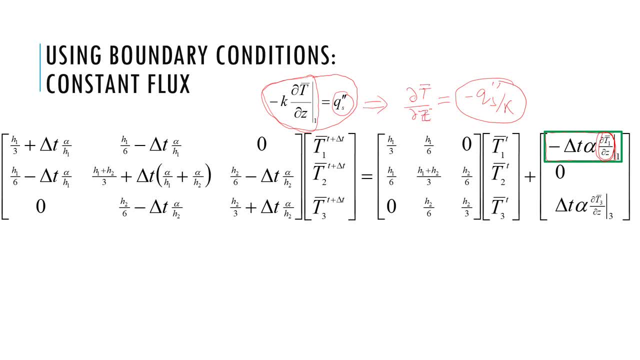 so if we replace that for del t, del z in here we are done. so let's see how that looks. so we just replaced that by this and and so alpha, as you know, is k over rho c p. so this k here that is coming from here would cancel with this k. so i get qso or we can even show that in here. 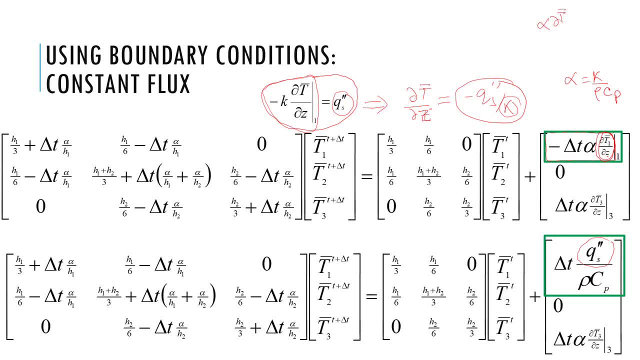 so alpha del t del z is equal to k over rho c p del t del z, like i said. so this part of it is equal to qs, or qs negative of qs. okay, so we plug in. so then this part is known. it's now known. so that's how we do. 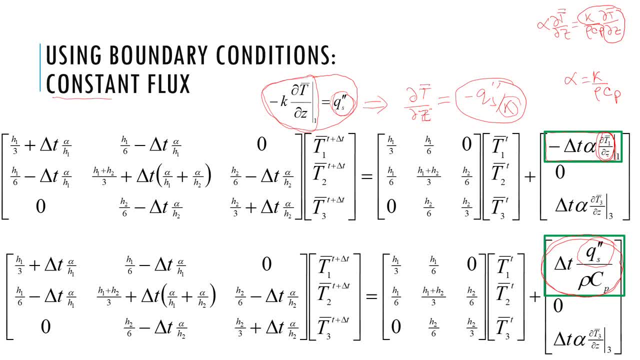 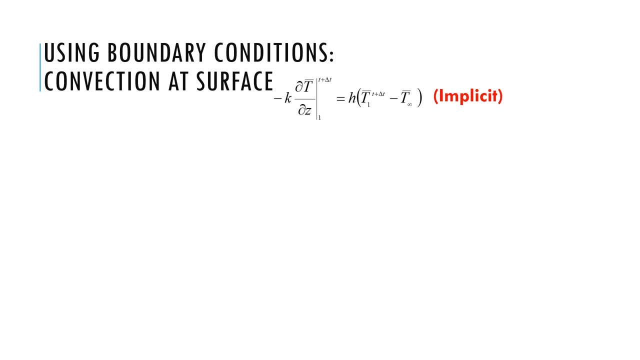 the, the flux specified boundary condition. then the last one is using convection boundary condition. so this is how we write convection boundary condition and we can choose to write this in a implicit way. we don't have to get into the the details now, but we could choose as t or t plus. 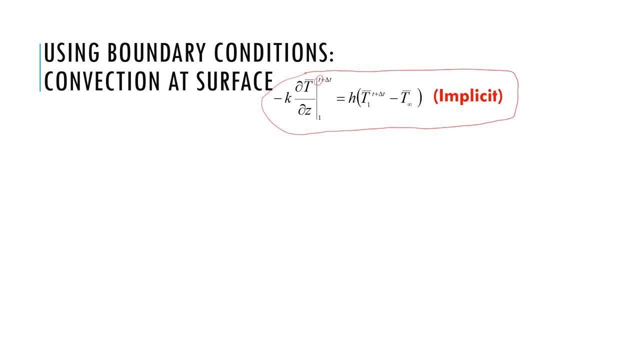 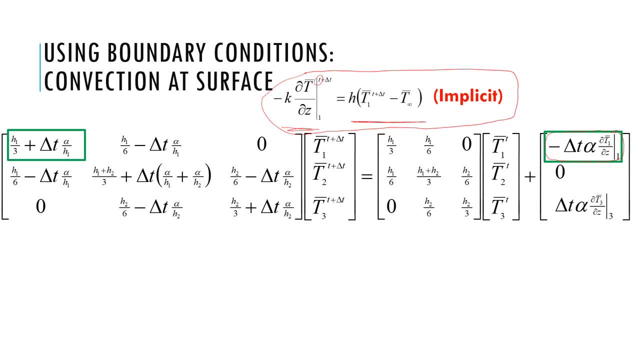 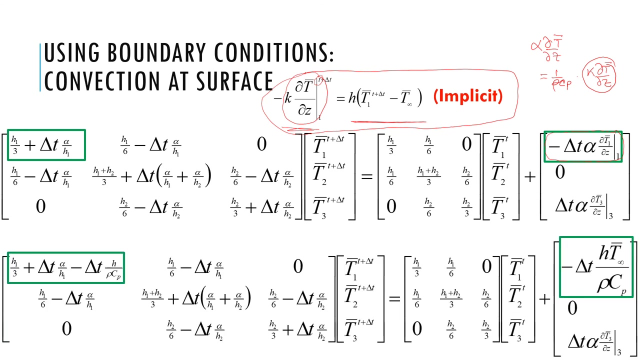 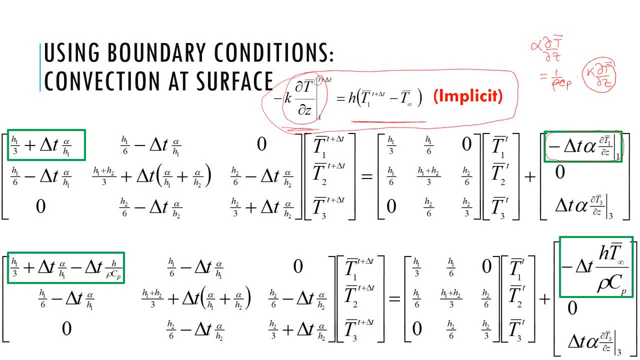 if we do a little bit of simplification, then this term changes to this. so all of these things are known. now H is known, and then T- infinity, the boundary temperature. this is something that is known, so this is now known. okay, so the that is how we handle the three types of. 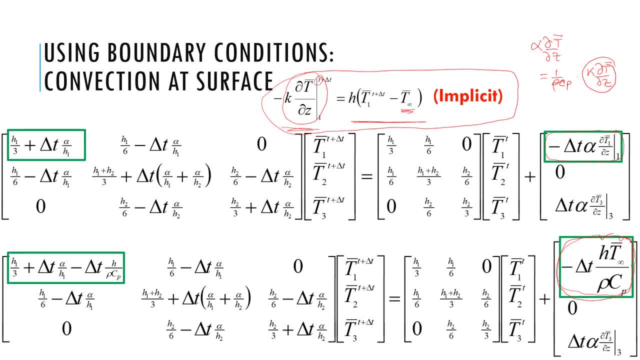 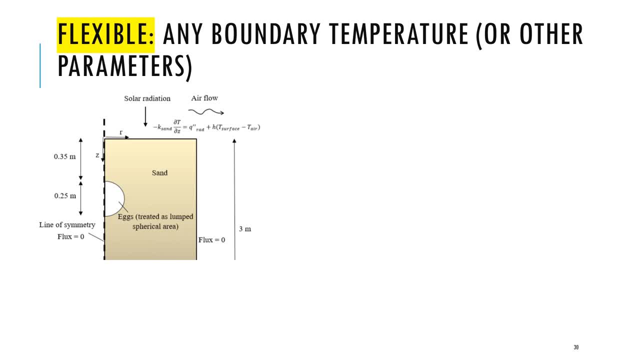 boundary conditions. one of the most useful aspects of numerical solution, like the finite element method, is its flexibility to use many different boundary conditions. for example, the boundary condition- the temperature surrounding temperature- doesn't have to stay constant, and I'm going to show you an example of that. so here is a 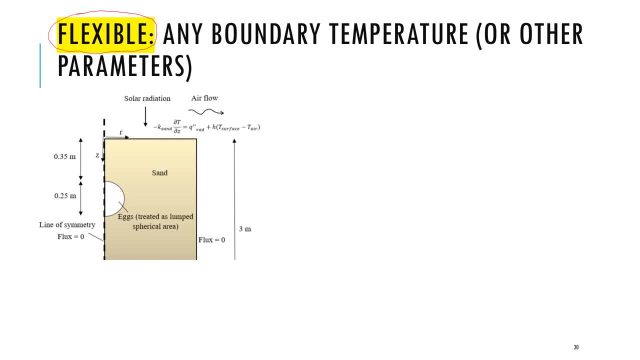 problem. okay, see, here is an example of a project from our class from the past, and the project has to do with hatching of eggs, total eggs in sand. so the eggs are at about this level and it's in the sand and there is some heat flux from the. 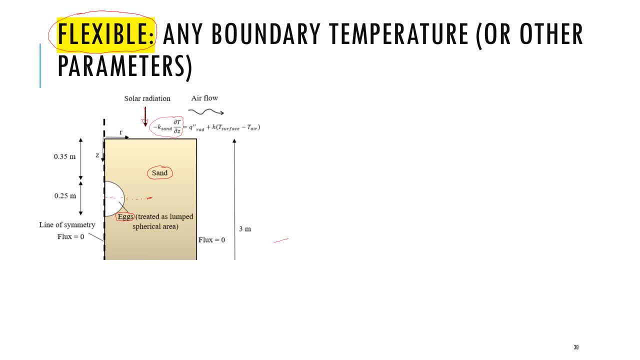 the heat flux at the surface. and why are we interested in the temperature? it's because whether the eggs will hatch into male or female depends on the temperature history that the eggs go through. so that's why we want to calculate the temperature here. now, i am not. 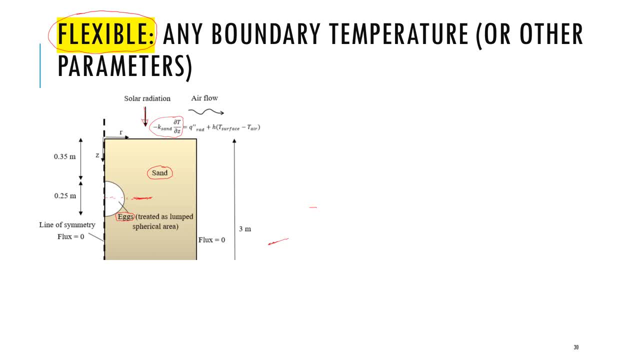 showing you all the detailed physics of this. i just want to make the point. let's say, i want to calculate temperature at this location. so without bringing in other complications due to, uh, the the egg being different from the sand and so on, let's say i just want to calculate. 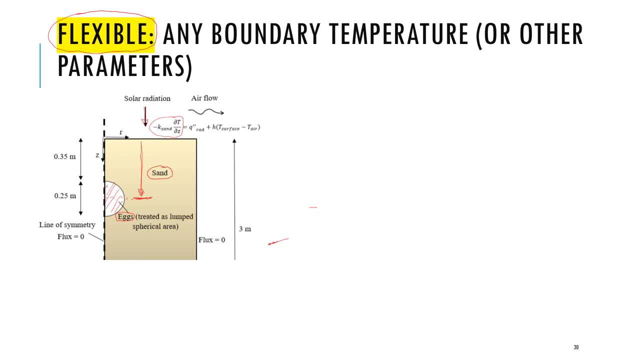 the temperatures here and um the. the problem is in this boundary condition, in this convective boundary condition, the temperature of the temperature, of the temperature of the temperature condition. let's get rid of the radiative flux part. so in the convective boundary condition, this air temperature is not a constant. in fact, it looks like this: this is the air. 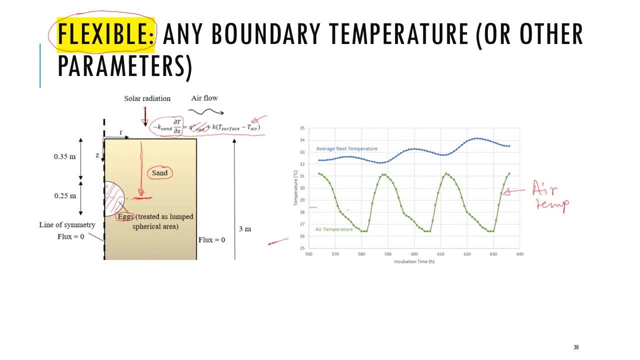 temperature. so if the air temperature keeps changing with time, how do i calculate the temperature here? by the way, the the solution looks like this: the average nest temperature. but how do i calculate that? i'll show you in next slide. it is hard to do this analytically, so here: 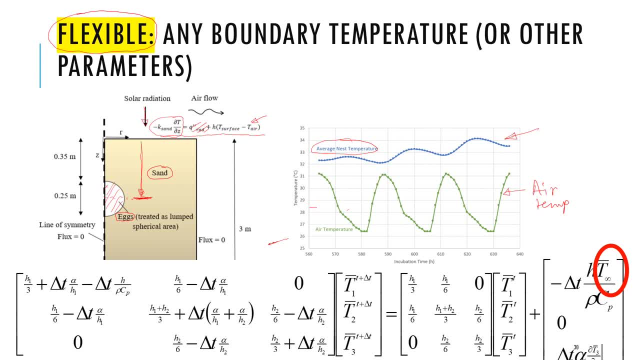 with the finite element method. this is very easy. again, i am showing these equations because we derive them. not that these equations apply to this problem, but the form of this is certainly the same as would be for this problem. i want to draw your attention to this part that has the t infinity. okay, 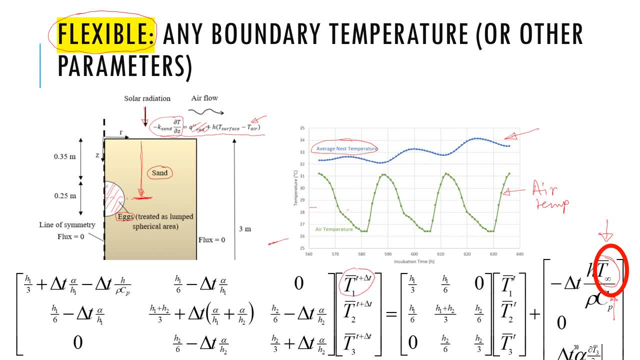 so when i'm calculating temperature at time- t plus delta t- so let's say this is my t and this is my t plus delta t. so when i'm calculating the temperatures here, i need the air temperature temperature so i can use the air temperature from here. for example. i know this temperature, so i use. 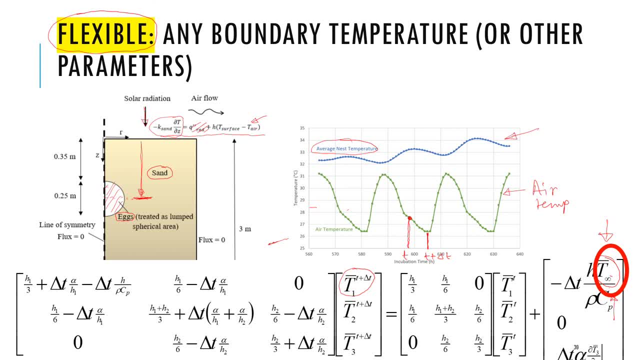 this value and i, by using that, i calculate temperature at t plus delta t. then the next time when i'm here and i'm calculating at t plus 2 delta t, here i just need to update. this is the only point for all the discussion. is this t infinity? it's the discrete value that is needed. 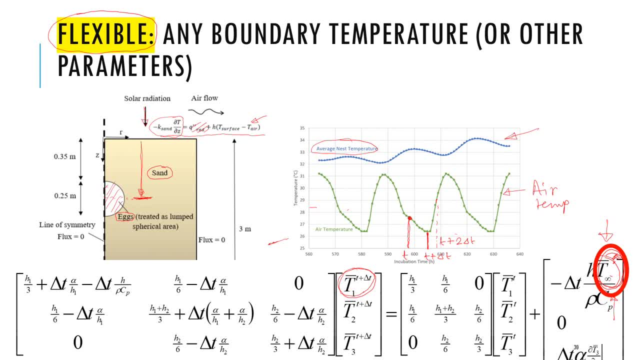 just for that time step, for that calculation. so when i am calculating at this time step, i just substitute the value here at the previous time step. so in other words, i keep updating, keep updating this value here and you, the temperature automatically will be calculated for these conditions. in fact, you can see that. 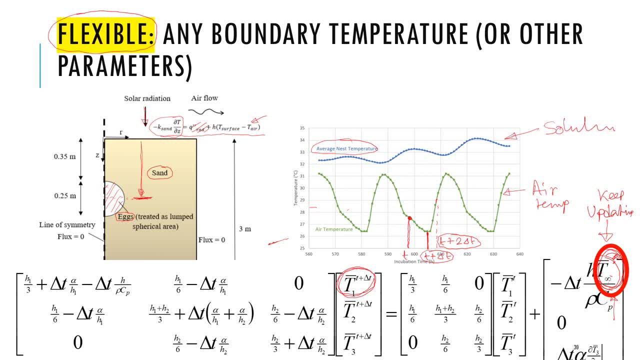 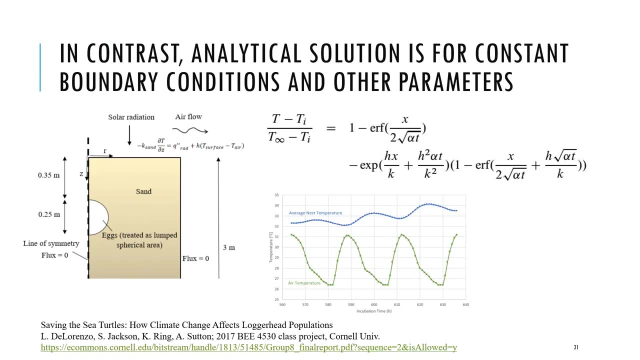 so you can see the solution. and that was calculated by changing the t infinity continuously, like this. so you? so this is not possible. for example, if you contrast this with analytical solution, this is not possible because so for the condition of a convective flux given, okay, for this condition in a semi-infinite region. 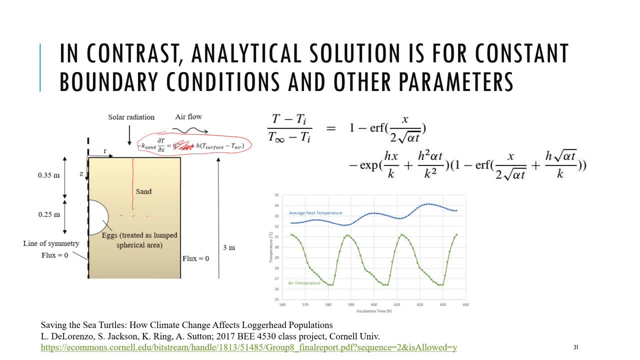 i can calculate temperatures using analytical solution. okay, so this is very possible. except this assumes t infinity to be constant, so t infinity has to be constant here. t infinity cannot be this, so this analytical solution is not flexible. means that t is constant, so let me write myself. 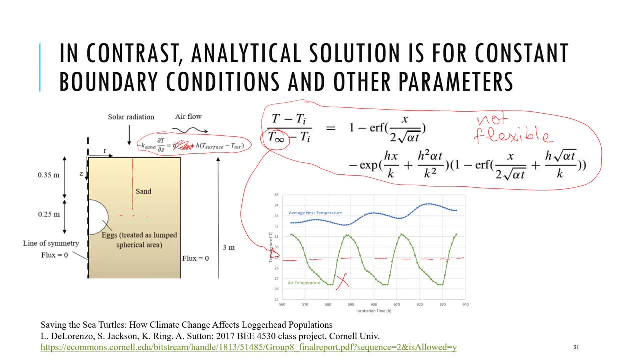 so i subtract t z inside iallah number plus i, i Article involved in it, with T infinity of course. second time different. so this is the first time for such move with T infinity, so that into x and x and y as the negative look, because the basic of it is the advantage of a. numerical method, like the finite element method, that it can track a, let's say, in this example, boundary conditions, for example. that can vary anyway. it may give you different measures. you get well, taken first. then we are just going to Santos, for example, and then do these both. but you stop training this and at the end you will likely have to unpack the approximation and help me to provide simple murdered elliam and with first the takea, which was right here, and then when merce Отp's in the same example. you don't seem to display this. you'll see that hiding in our 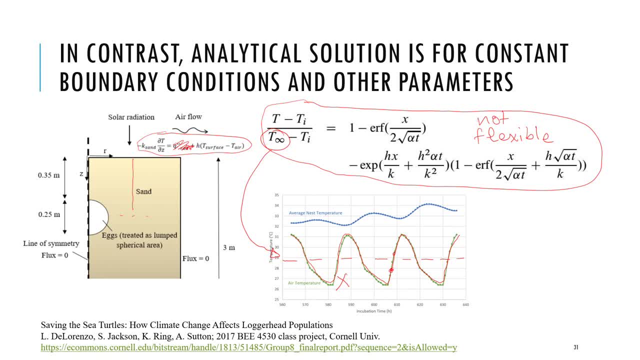 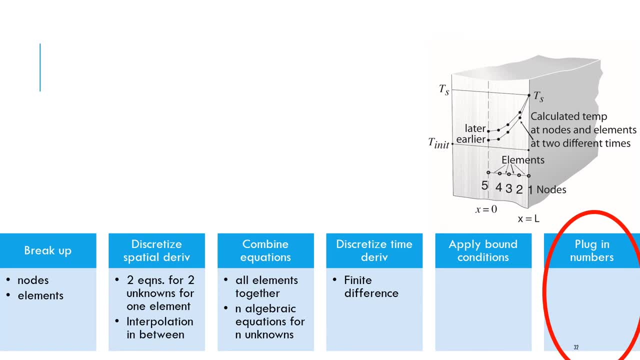 it wants. we just need to know what it is, that's all, and then we can use it. so this final step is not much else we're done, but we just want to plug in numbers and just to make us feel comfortable with the final product that we got. okay. 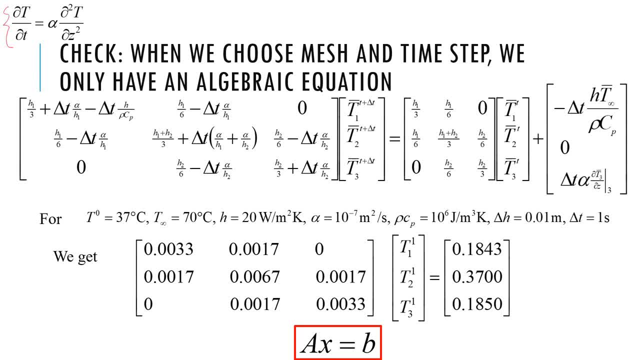 so this was our original governing equation, the heat equation, and we converted it from the differential equation to a set of algebraic equations. okay, so, even though it's algebraic equation, you know, with all these symbols everywhere, it may not be obvious that we have achieved something really great. we. 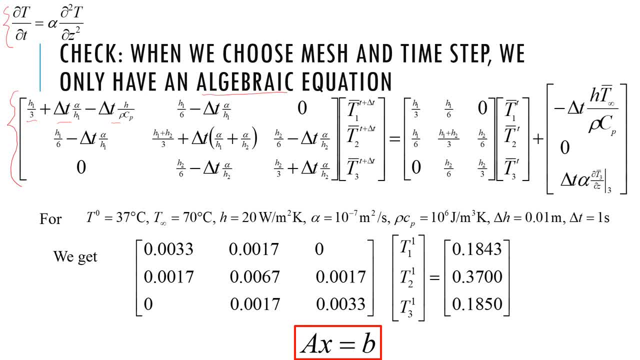 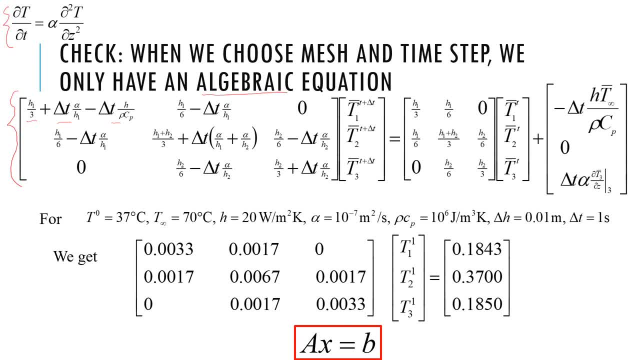 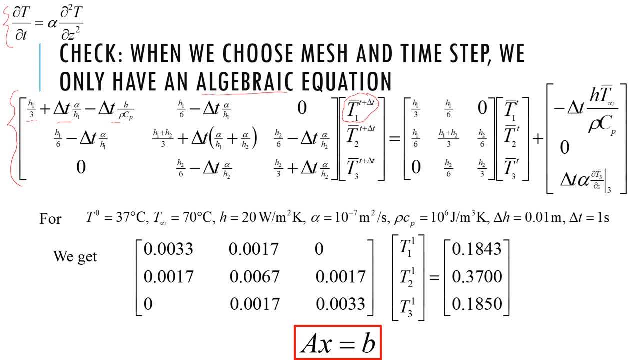 temperatures at time, T plus Delta T. so for an initial temperature of 37 degrees, ok for T infinity. the ambient temperature of 70 degrees H, the heat transfer coefficient of 20, the thermal diffusivity of 10 to the minus 7 meter square per second. density, time-specific heat as 30. 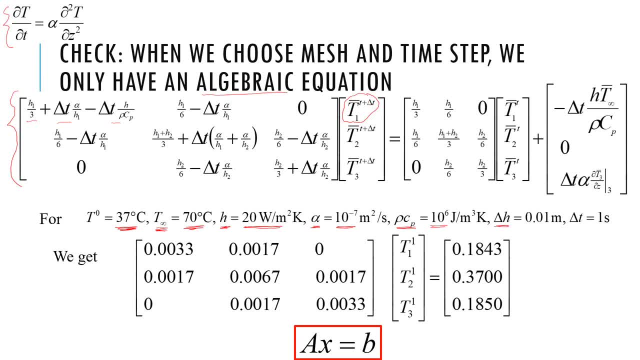 10 to the sixth, Delta H. this is the. you know we are doing this for a slab and so we are dividing the domain from the line of symmetry to the surface. We are dividing it into a number of nodes. So delta H is the size of the element, which is same as this H1.. So we choose that and 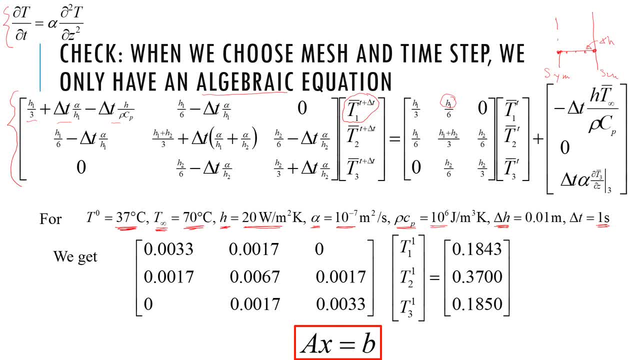 we choose one second time increment. So if we choose all this, then we plug in to all of these values. then it looks like this: Now would you believe that it's an easy thing to do? So we just have to solve these three equations. 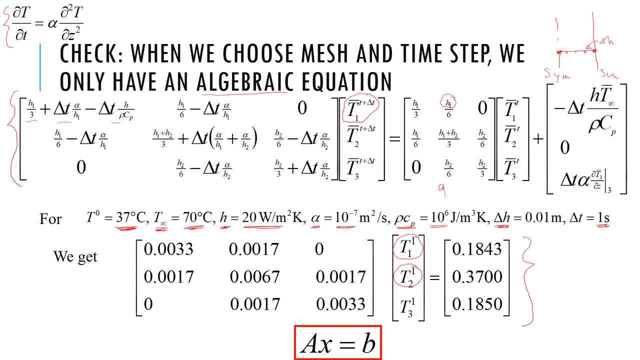 For the three unknowns temperatures at the three nodes at time step one, And then this would be used to calculate the time step two, T2 or T1 at two, that will go to T1 at three and so on. So at 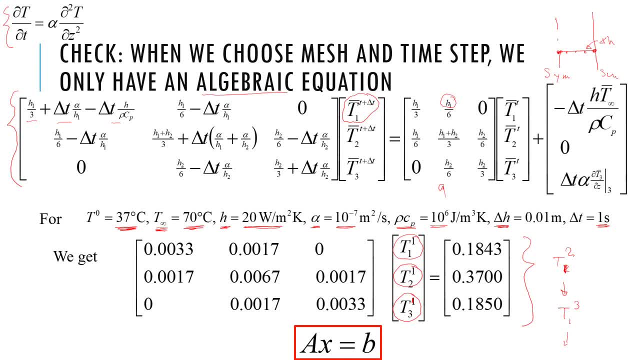 different time steps, And so it's really easy. It's a simple process right now. Now, of course, very large systems of equations. It's not simple, but at least conceptually. you know we have gotten completely out of the PDE solution to. 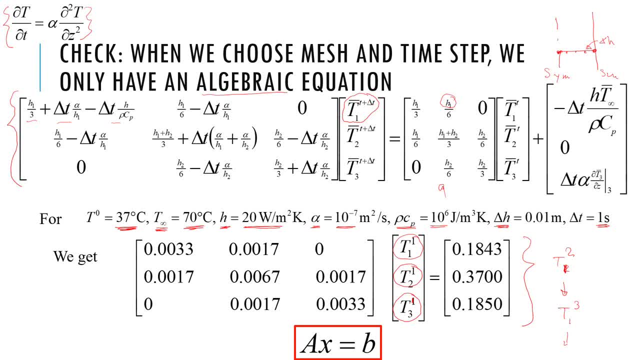 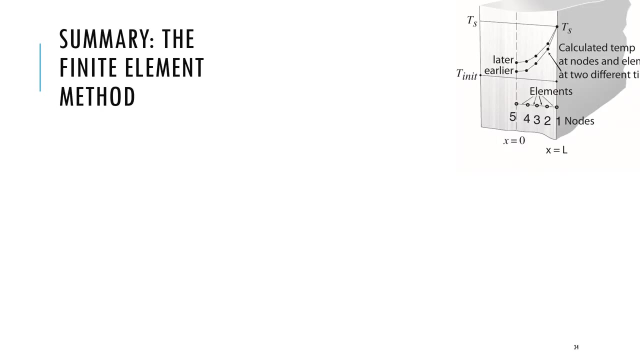 solving a set of linear equations where these are the variables that we'll solve for. So the form of it is our, you know, most common AX, X equal to B. So we solve for X. So we now summarize everything we did in this building up of the finite element method. 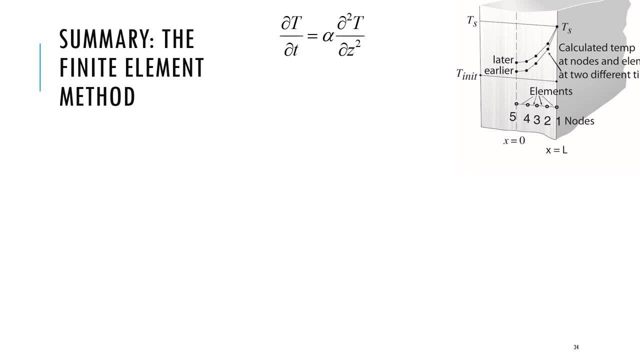 So first is we took the differential equation and converted into algebraic equations And we did that. That is the process Of building the finite element equations And we did that by first breaking up the domain. So the domain in this problem, in this is this: the thickness of the half slab. 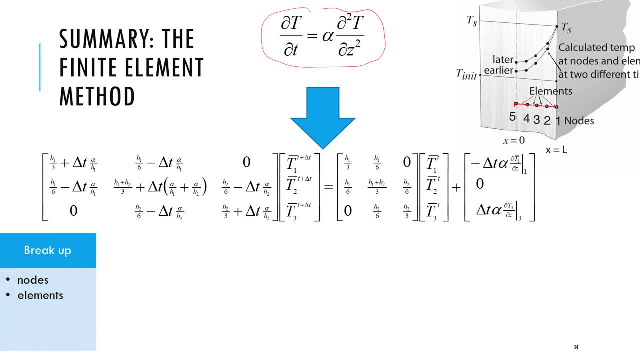 It's symmetric, So we need only half slab. So we break it up into nodes and elements. That was the first step. Next we discretize the spatial derivative here for one of the elements. So we did that And then we combined equations for all the elements. 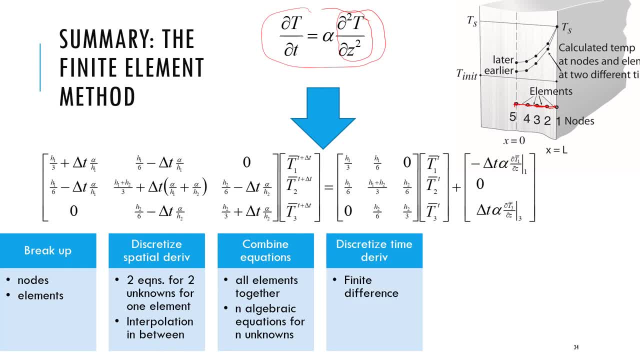 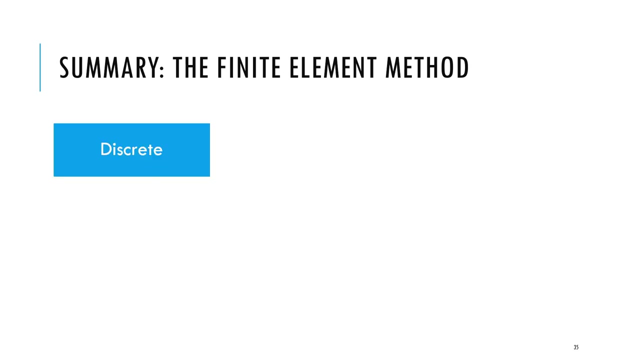 And then we discretize the time derivative, And then we applied the boundary conditions And that's basically it. And then we plug it in, And then we plugged in numbers just to see how things go. So there are some very important points worth noting of this method.